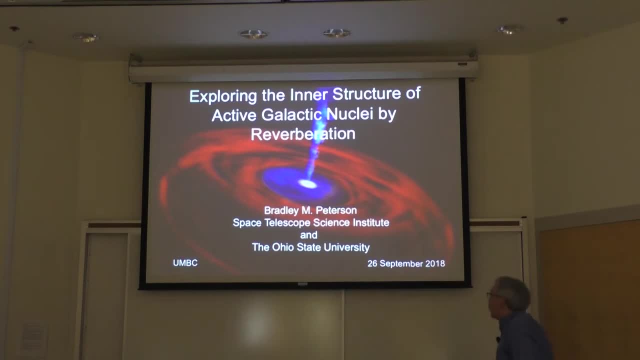 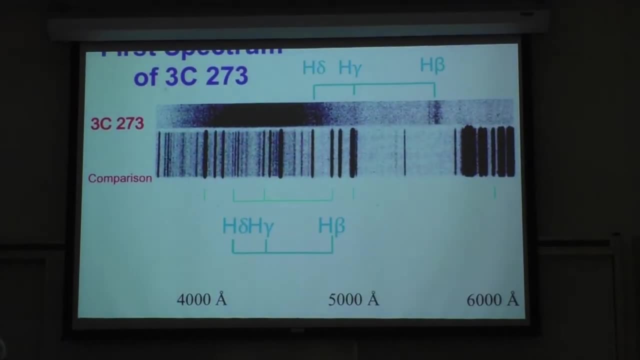 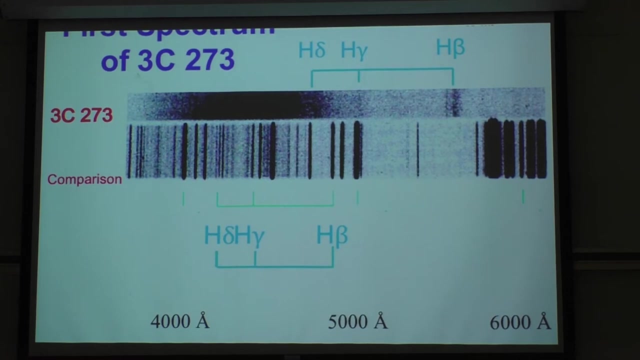 my visit very much Okay. so let's start out talking about quasars. What are they? Well, the quasars were first identified about 55 years ago. First, they were radio sources that seemed to be associated with star-like objects on the sky. They were distributed all over the sky. 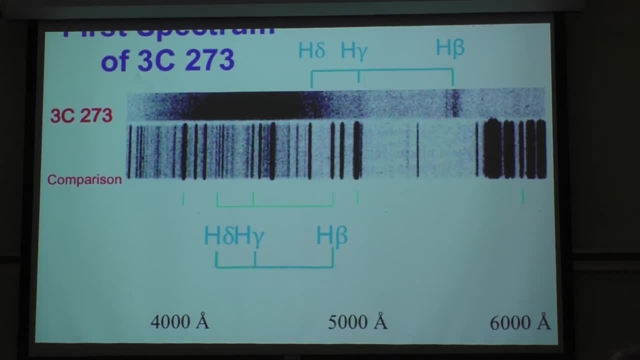 so they appeared to be not galactic, but they appeared to be star-like, unless you looked at them very carefully. If you look at them very closely, you will see- I'll show you this in the next pictures- that sometimes they seem to have some kind of halo or fuzz around them. In fact, in the Astrophysical Journal you 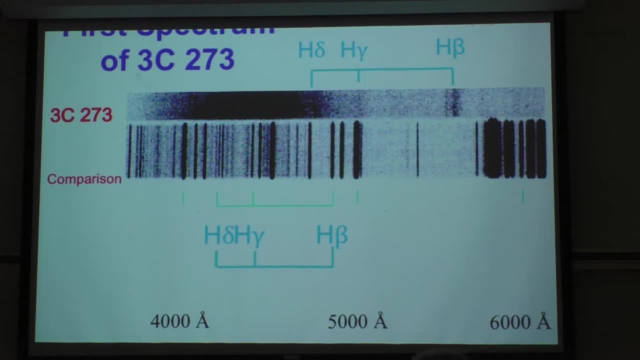 could find articles written about quasar fuzz. Studying quasars in the early years was an art, largely because of the kinds of detectors that we were using. We were using photographic plates to obtain spectra. So this is the description of a quasar: It's a quasar and it's a kind of a. 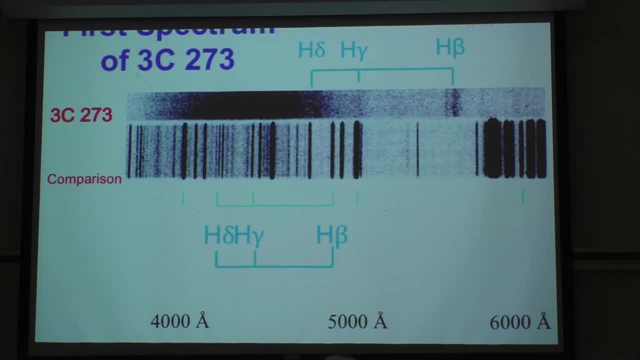 discovery spectrum for 3C273.. And you can see it's a negative. so where it's dark, you're seeing light And you can see that there are these emission features. Let's see, this is not a very good laser pointer. Do you have another? is there? Oh, I'll make two. All right, You can see where. 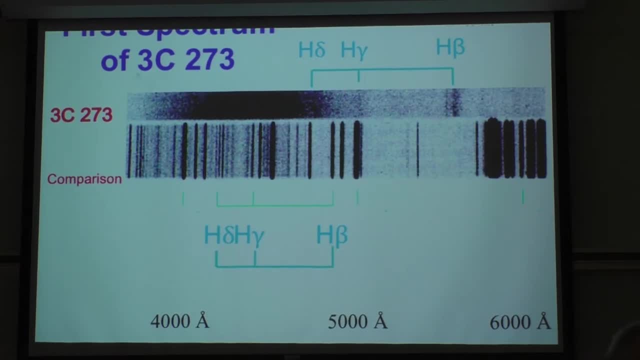 the Balmer lines are labeled. Now, it took Martin Schmidt a while to actually figure out what he was looking at. It's a familiar pattern in the distances between the lines, but it took him a while to sort of wrap his head around the fact that it was the Balmer lines, because they were significantly redshifted relative to their laboratory positions. So, again, this is a. the comparison spectrum, then, is simply an arc lamp that provides you a wavelength calibration, and the spectrum that you see on top is the quasar 3C273. 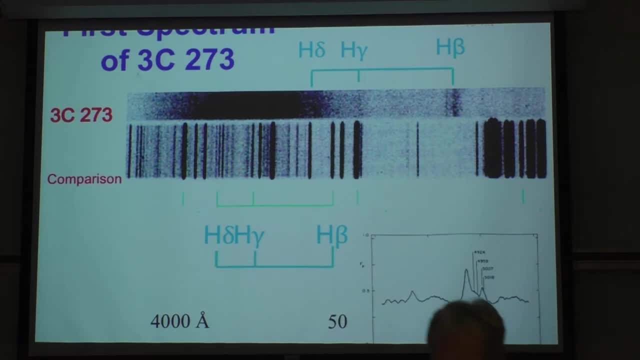 I did the laser pointer. Oh, you did wonderful, Great. Don't let me wander off with it, Okay. Okay, it's smarter than I am. There we go Pulled the wrong way. God, that hurts. Okay, This is a more modern spectrum. taken with a linear detector, You can see these very broad emission lines. That's a characteristic, then, of quasars, or what we now call more generically active galactic nuclei or AGNs. So it's actually. these broad emission lines are going to figure very prominently in what I have to say today. 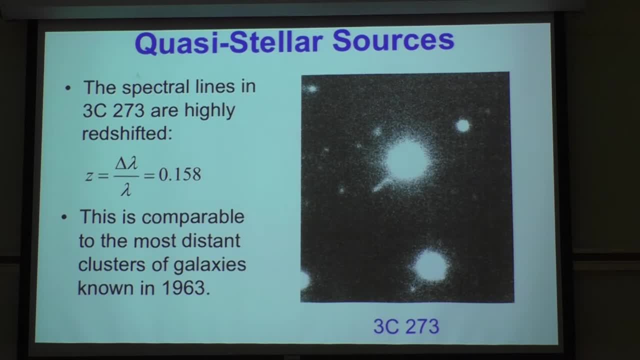 So if you look at quasars, they seem to have extended emission around them that was known as quasar fuzz. We now know that this is starlight from the host galaxy that the quasar resides in. Now, the reason it took Martin Schmidt a while to sort of wrap his head around the fact that this was highly redshifted Balmer emission was simply because the redshift was about 16%. 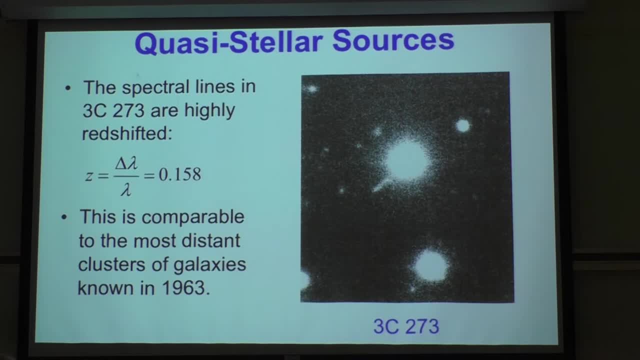 Now there were distant galaxies that had similar redshifts due to the expansion of the universe, but the most distant galaxies known were a comparable naval, terrible redshift to this, but they were the brightest galaxies in clusters of galaxies. And this thing- this 3C273, is a hundred times as bright as the brightest cluster galaxy. 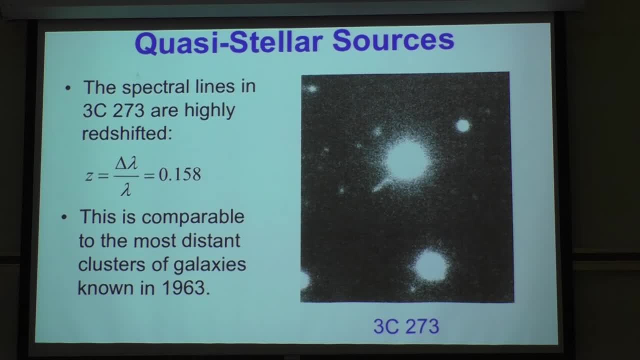 So that's kind of interesting, right, because the brightest galaxy in a cluster is the light of nearly a trillion stars, and this is a hundred times as bright. So it was again. this is something that was very challenging to try to understand in 1963.. 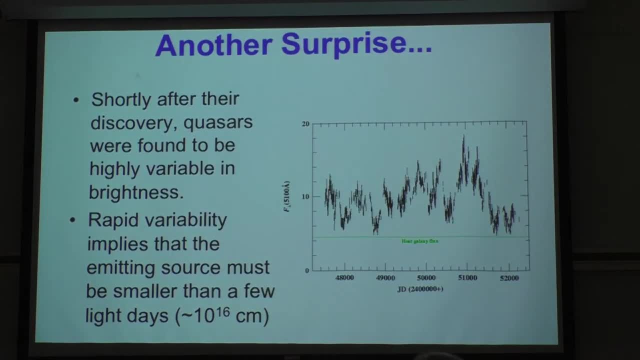 Okay. so shortly after this discovery, there was another surprise. People started to look at these things again and again to see if their brightness changed with time, and they discovered that the brightness of quasars changes very rapidly on short time scales, indicating they must be physically very small if the source is varying coherently. 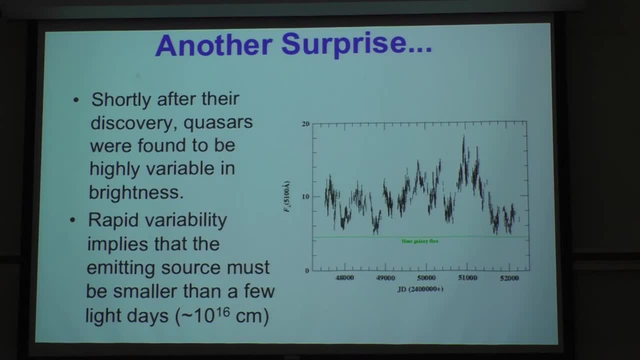 So the limitations on the size were a few light years, Light days at most, in other words, something less than around 10 to the 16 centimeters or so. So what you have is an object that's a hundred times as bright as the brightest known galaxies. 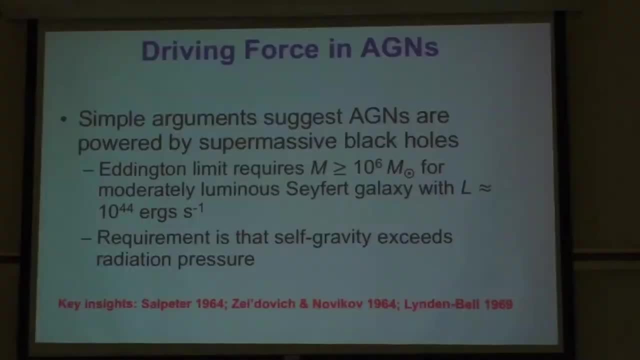 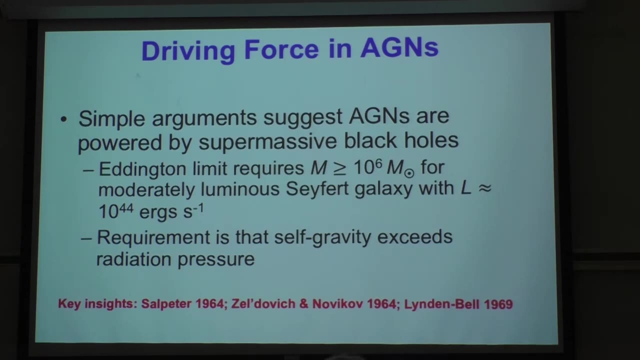 and it's contained in something the size of about the solar system. Okay, so this immediately suggested that it might be that gravitational accretion could power these things, and it would have to be done by supermassive black holes. Why supermassive black holes? Well, there is a limit called the Eddington limit. It's how massive a thing must be to keep its radiation from disintegrating it. So this is a limit that you find. This is one of the things that limits how massive stars can be. As stars get more and more massive, they rapidly become more and more luminous. They increase in luminosity with mass faster than they increase with mass. So once you get up into the range of hundreds of solar masses, the radiation pressure becomes so much that it beats gravity and blows the star apart, or keeps it from forming at any rate. 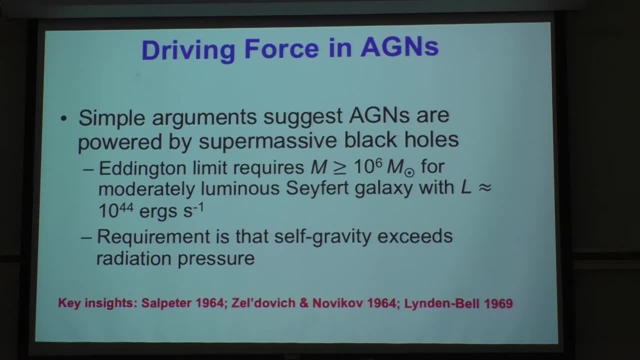 So if you apply this Eddington limit to massive objects like well, to objects like quasars, you discover that they must be massive. They must be for a typical Seaford galaxy, which is a low luminosity agent. 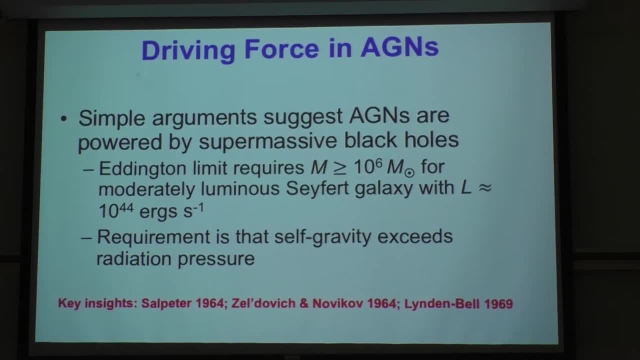 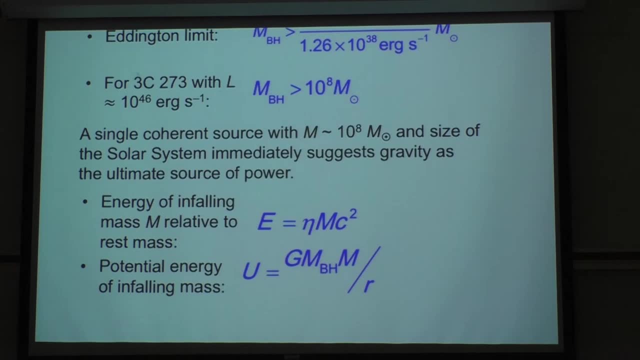 they have to be larger than about a million solar masses. So now what we're looking at then with 3C273,. oh, we lost a little bit on the top there. I Eddington. anyhow, That's the Eddington limit on the right-hand side. 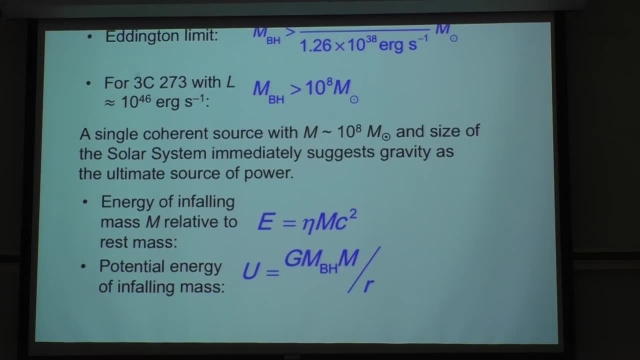 Is there any way we can rotate that down just a tad? No, OK, well, we'll just roll with it then. OK, I will tell you that the numerator on this equation is the luminosity. So with 3C273, which has a luminosity of 10, to the 46 ergs per second, 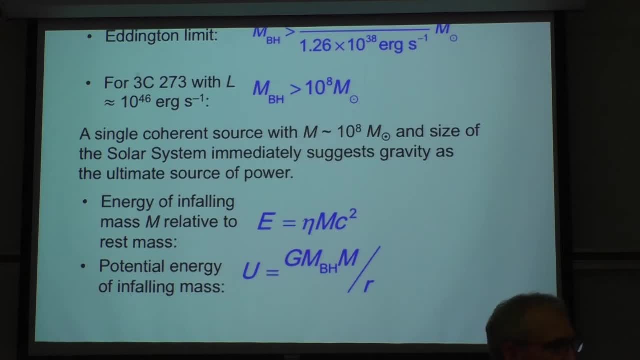 assuming that it's at the distance indicated by its right shift, that tells you that it has to have a mass larger than 100 million solar masses. This is pretty large. Again, this suggests that it must be gravitational accretion that must be the source of the energy. 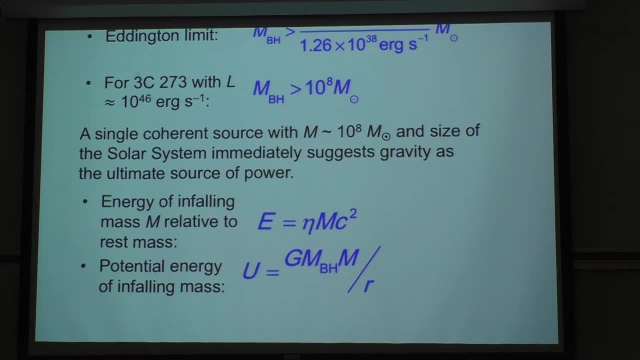 So let's actually work through that in sort of an order of magnitude way, the way astronomers like to do things. So let's express the energy that we can get from a particle dropping into a deep gravitational potential in terms of its rest energy. so the energy of the particle is going to be some. 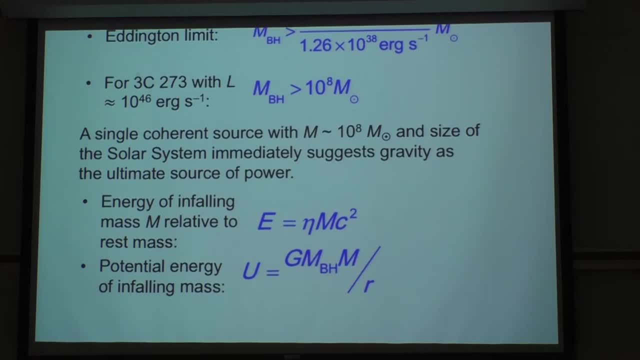 eight of an inch, I think, which is an efficiency times mc squared. So what we want to do is figure out how big eta is. So the potential energy of a mass at a distance r from a black hole, m sub bh here. 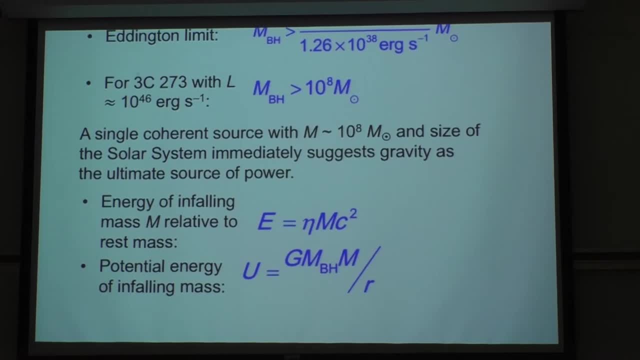 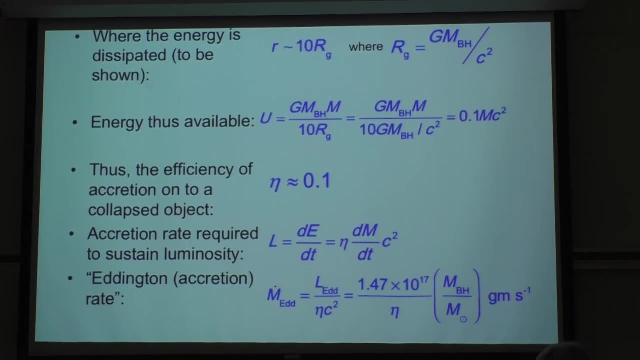 potential energy is given by the lower equation, very simple one from freshman physics. Now ask yourselves: where does the particle have to fall as it falls into the black hole? at what point does it dissipate its energy? And I'm going to assert for right now. 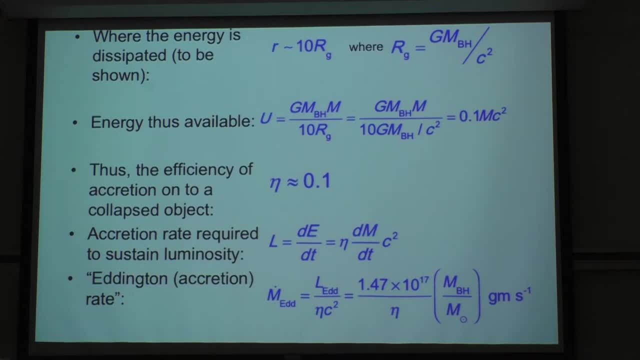 that it happens at about 10 gravitational radii and then demonstrate that later. So we've got a number that occurs at 10 gravitational radii. So the amount of energy that's available then works out to be, if you plug that into the potential energy equation, a tenth of the rest energy. 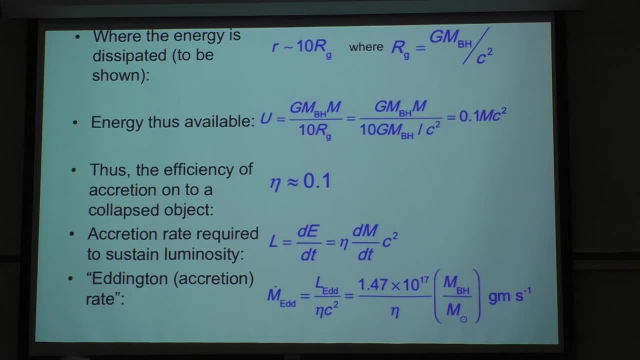 So the efficiency then is 0.1.. This is much larger than the efficiency of converting hydrogen to helium, which is 0.007.. So this looks like a potentially fruitful thing to look at. So if we want to sustain the luminosity equation, 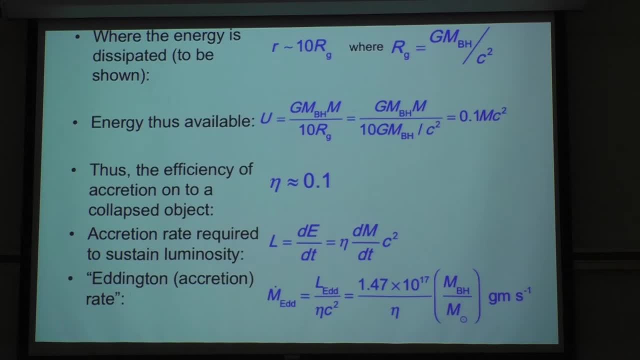 we have to dump in mass at a certain rate. So we'll take that equals eta mc squared equation. then take the time rate of change of that and that gives us the luminosity ergs emitted per second, or watts. sorry. 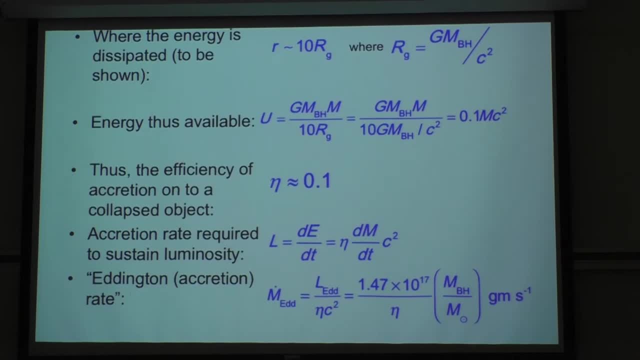 I'm a physicist, I keep forgetting they're using watts when we're mired back in ergs per second. Okay, so luminosity then goes like eta times, the mass accretion rate, times c squared. So we also define an Eddington rate. 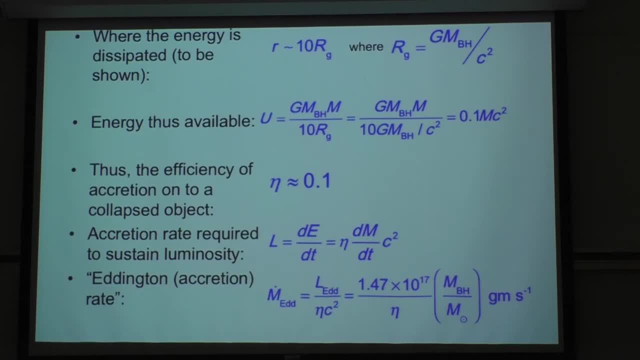 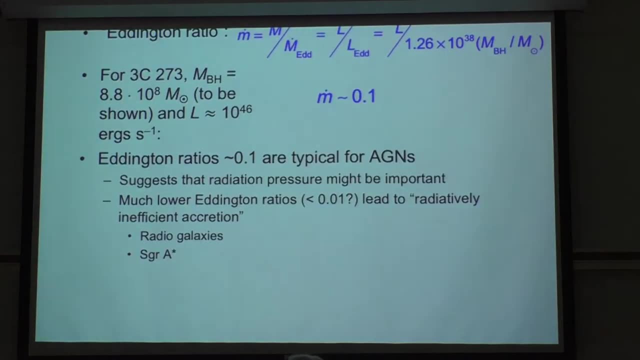 and the Eddington rate is the rate at which you would have to accrete mass onto an object to reach this Eddington limit, And that's given by the lower equation. Now we're really interested in the ratio of the real accretion rate to the Eddington rate. 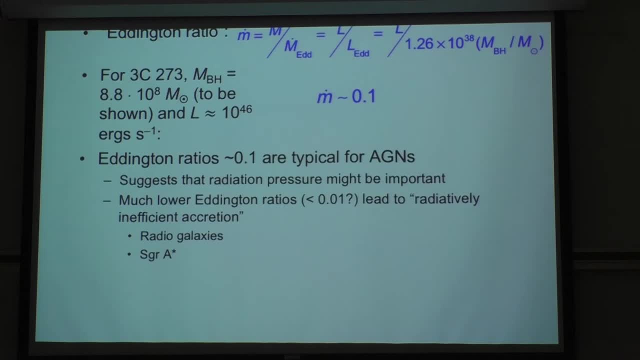 which we call the Eddington ratio, And that's given by the equation on top. And for 3C273, its mass turns out to be- and this is what I'll be showing you how you get this later- nearly a billion solar masses and with luminosity. 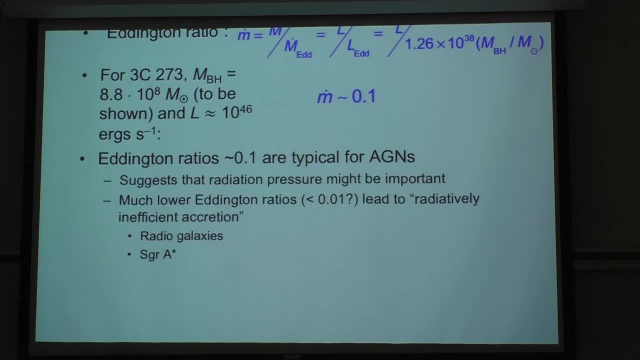 of 10 to the 46th ergs per second. that gives you an Eddington ratio of about a tenth. Eddington ratios of about a tenth are typical for active galactic nuclei. It also suggests that radiation pressure might be important. 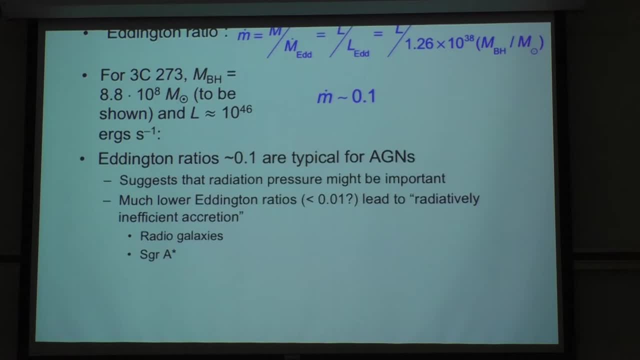 because the rate is not. it's an order of magnitude lower than the Eddington limit, but it still might be there. And it turns out that much lower Eddington ratios below a hundredth or I think, actually below .0001,. 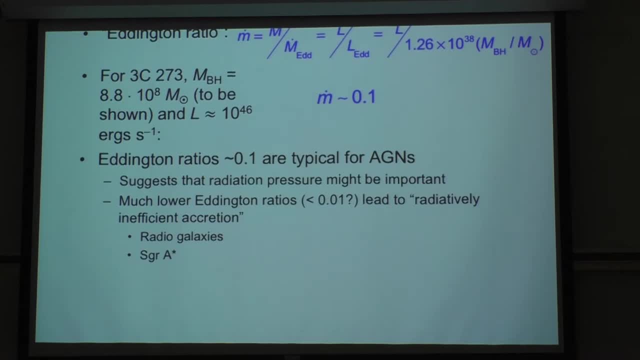 read more about it. It leads to radiatively inefficient accretion. This is the kind of thing that we have in our own galaxy, with the center of the galaxy a source known as Sag A star and sources that we see in what we call radio galaxies. 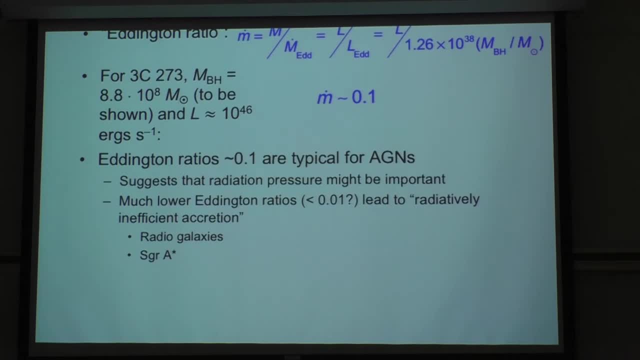 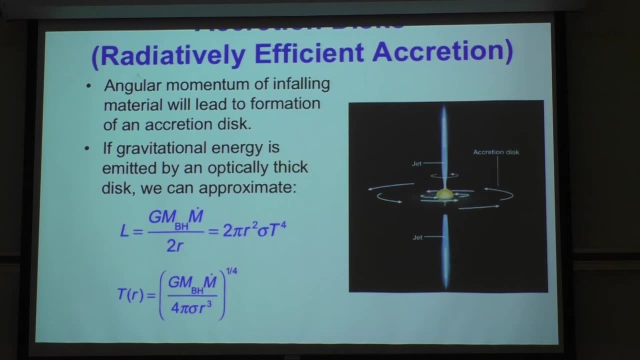 These are black holes that are accreting at much lower rates, So the ones that accrete at high rates tend to produce an accretion disk. This is basically due to conservation of angular momentum. As material piles up near the black hole, it tends to form. 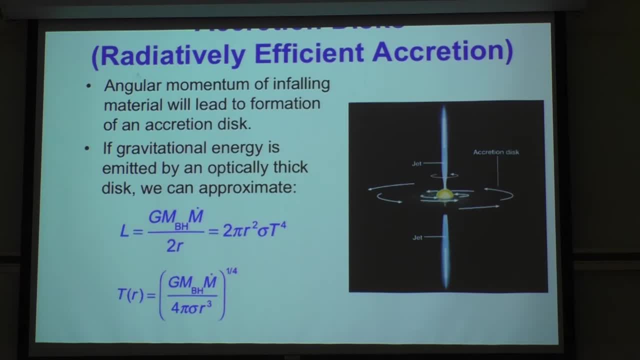 a rotating disk that is optically thick And the details of this are still poorly understood, poorly modeled, but we can get some again some order of magnitude understanding of this by setting the luminosity equal to half the potential energy. this is what we can get out of it. 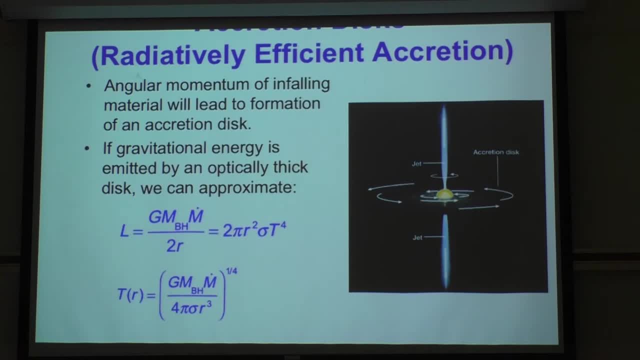 And we'll say that the emission is coming out then from an optically thick medium. So the Stefan-Boltzmann constant enters into this. we have that the radiation emitted per unit area is sigma times t to the fourth, and then we multiply this times. 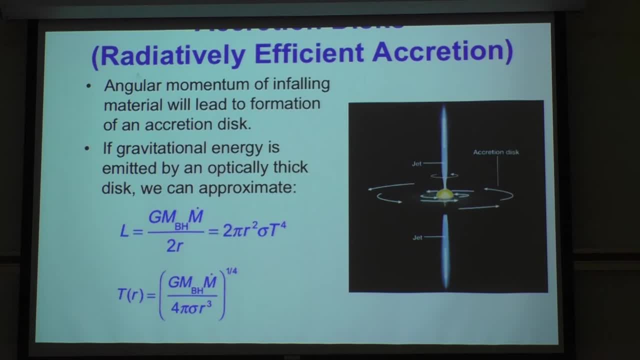 the emitting area of the disk, which is simply a circle, pi r squared. but a disk has two sides, so we have another factor of two in there. We can solve this in sort of an order of magnitude way for the temperature then, as a function of radius. 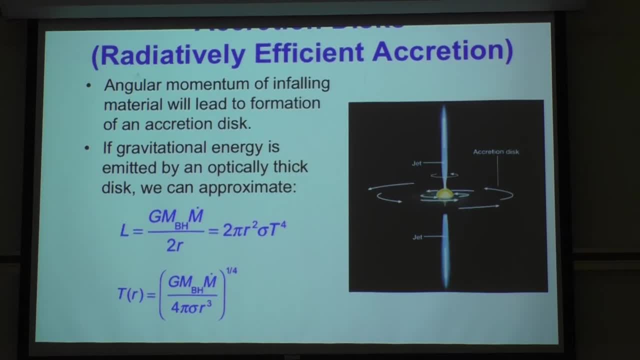 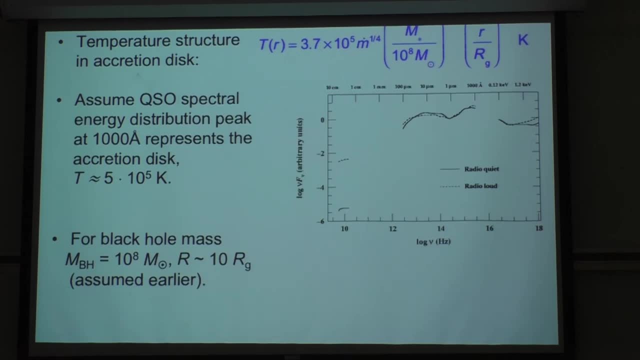 This gives us then? what is the temperature gradient of an accretion disk? and the temperature if I plug in all the numbers, as you see on top, and reasonably scale them, this tells me what the temperature profile looks like. And now if I look at the energy distribution from a quasar, 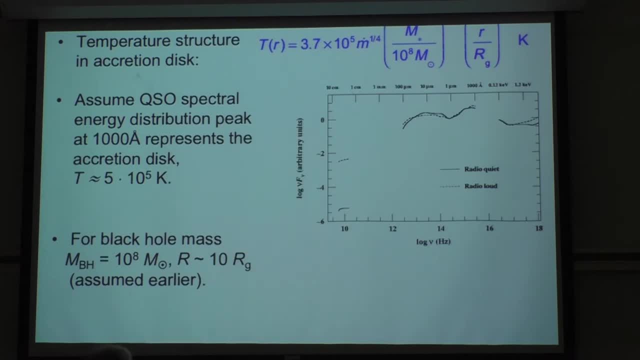 all the way from the radio on the far left to x-rays and gamma rays on the- well, just x-rays, I guess. in this case on the far right. what you see is that there are a couple places where the the spectral energy distribution is maximized. 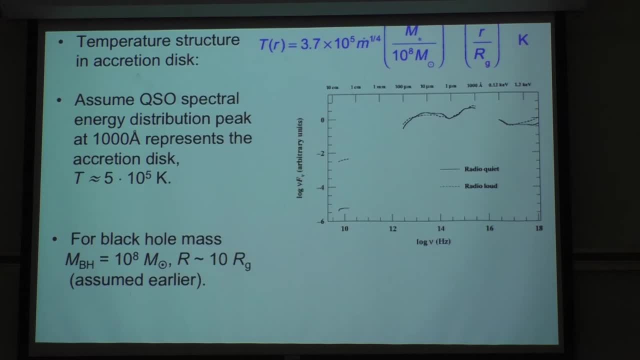 One of them is right here. this is the one that is supposed to be thermal emission from the accretion disk. Now we don't have any observations between here, between x-ray and UV at about 900 angstroms, because this is where the entire galaxy is opaque. 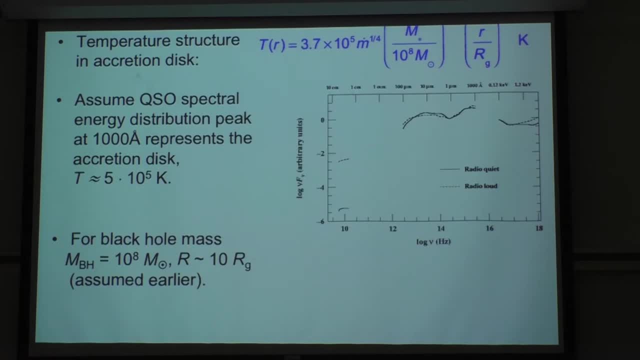 because of hydrogen in the plane of our own galaxy. So it's only when the cross-section for absorption becomes very low to ionizing photons that we can observe again. Anyhow, this appears to peak at about 1,000 angstroms. 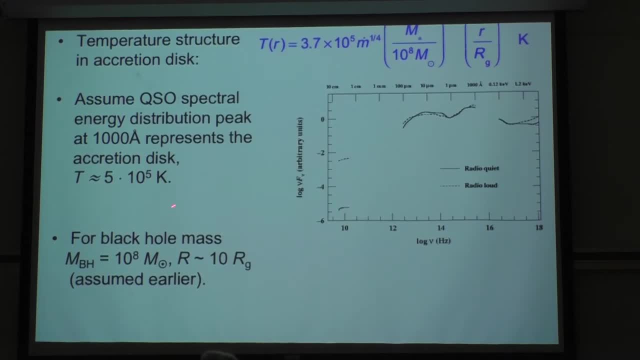 So if we just apply Wien's law to this, this tells us that the peak occurs at a temperature. well, temperature occurs at about 10 times 10 to the 5.. And if we work out where that actually is located, putting in that temperature here, 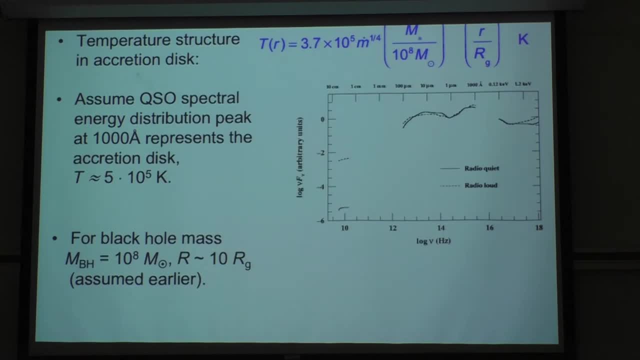 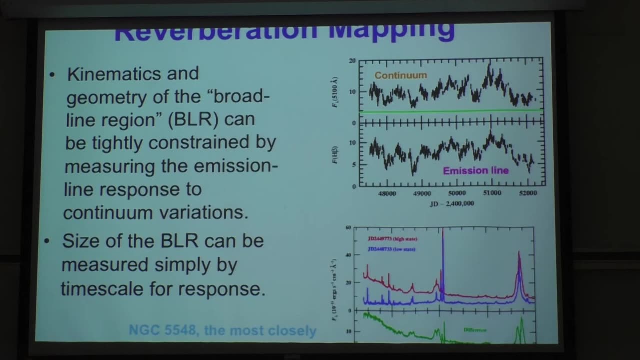 we find that that occurs at a radius of about 10 gravitational radii, which is what I was postulating earlier. Okay, so that's the basic physics of AGNs. Now I want to look at the inner structure of AGNs, And it turns out the light from the accretion disk varies kind of irregularly. 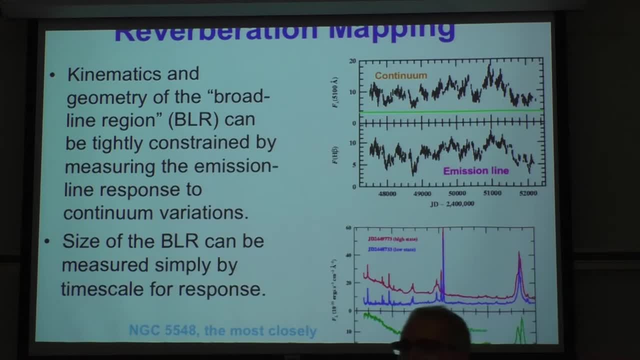 It's often described as a damped random walk, and the damped part means that just given an infinite amount of time, you're not going to see infinite excursions. There's some limit to how much it can vary, And this is if you look on the top diagram over here. 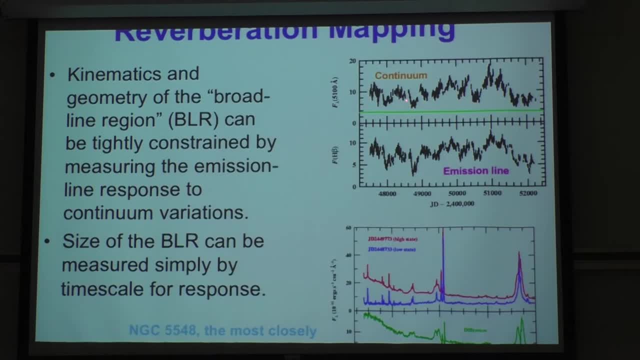 on the right on the top panel you see continuum variations over a period of about 13 years in one relatively nearby bright AGN that we'll figure prominently in what I have to say today. Now the interesting thing is if you look at the emission from the accretion disk, 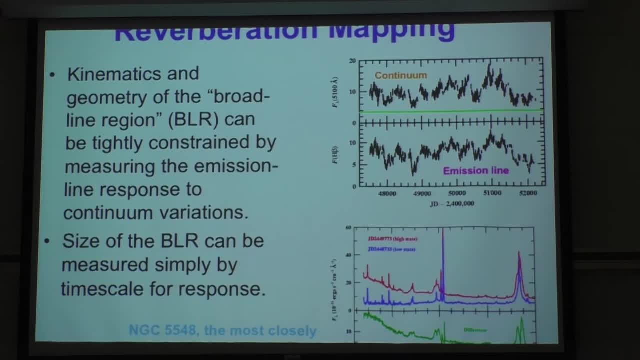 it varies with time. you also see that the light from the emission lines also varies with time, So it's clearly responding. the emission line gas is clearly responding to the light from the emission lines, So it's clearly responding to the changes in the ionizing continuum. 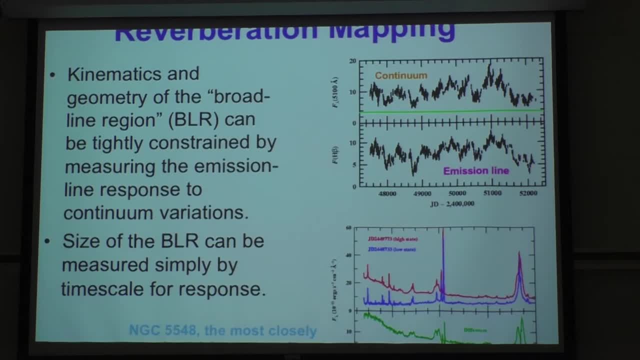 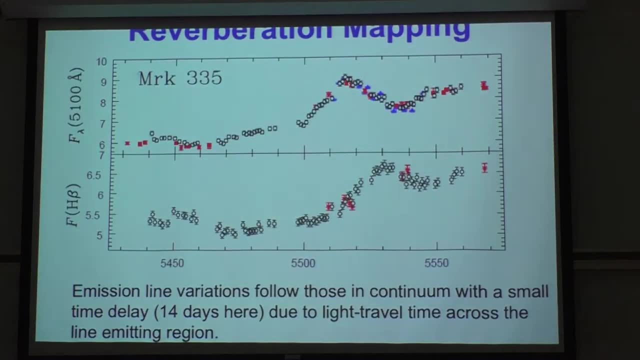 from the accretion disk and responds to those changes. Now the interesting thing is, if we look at this at higher resolution, higher time resolution, what we see is that there is a delay between the variations that we see from the continuum and the accretion disk. 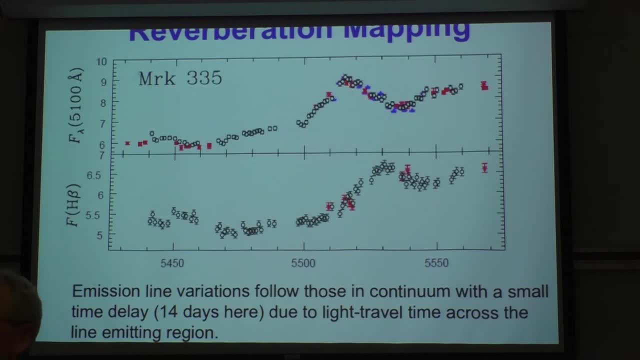 and the response to the emission lines, And this is due to the light travel time across the emission line region. So we have now a way of measuring the size of the emission line region just by doing simple cross-correlation of these two light curves. 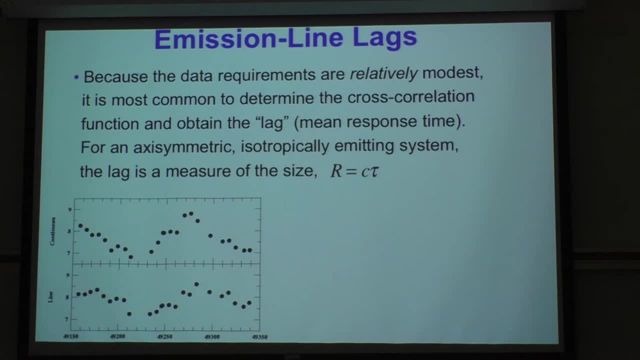 And if we do that, we find that you can even have a fairly sparsely sampled light curve. This is actually over an AGN that's observed over one observing season at a cadence of about once a week, And you can see the continuum variations here. 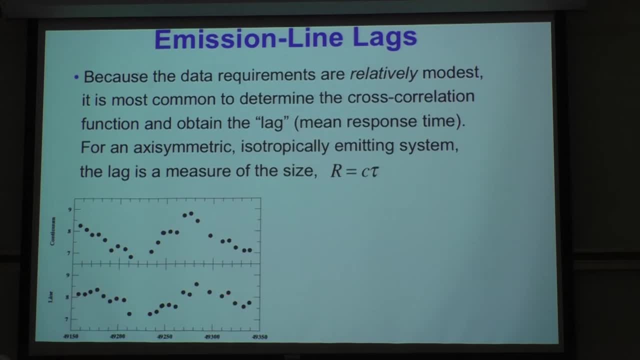 And here you see the H-beta emission line variations, which are slightly time-delayed, And if we simply cross-correlate these, we find that the typical size, a scale length, for this region is a little more than two weeks' time. 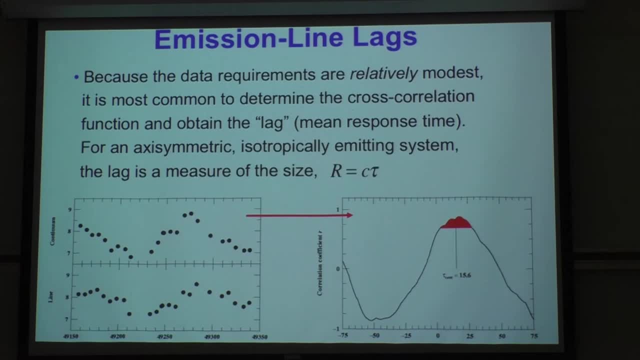 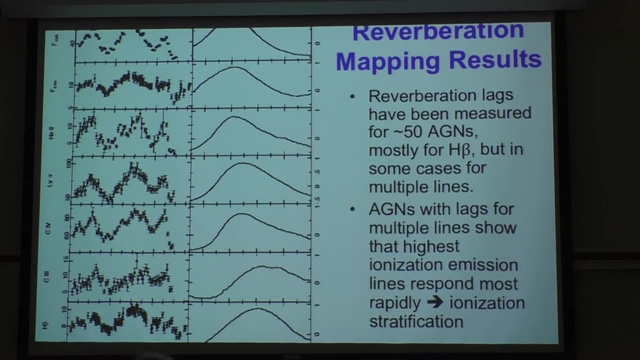 which translates then to a distance by multiplying by the speed of light. So if we look at multiple emission lines in a particular AGN, as you see here, this actually causes me some distress to show this slide, because until relatively recently this was our best reverberation data set ever. 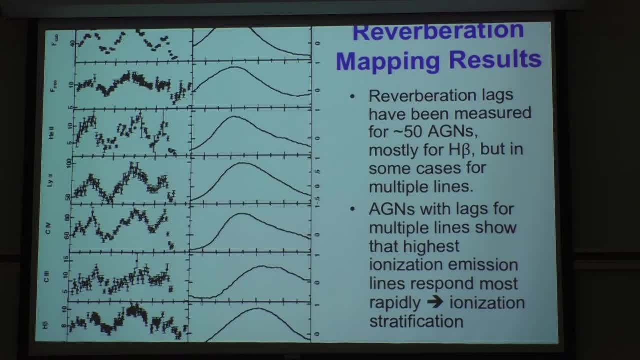 and it was taken back in 1988 and 89. It was largely taken with the International Ultraviolet Explorer, a small ultraviolet spectrometer that was a precursor to Hubble Space Telescope, And what we see up on top is the continuum variations in the ultraviolet 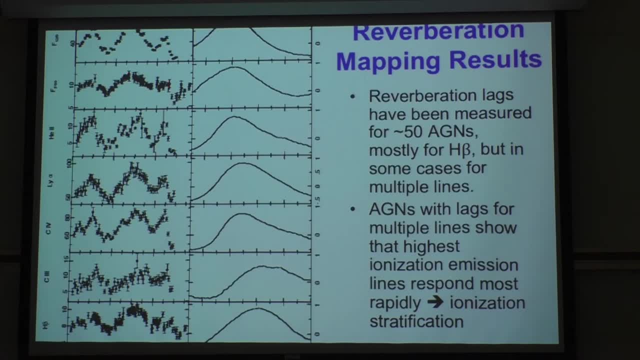 Immediately below this, we see the continuum variations in the optical part of the spectrum obtained with ground-based telescopes simultaneously, And now we can look at various emission lines going from helium-2, 1640, to Lyman-alpha carbon-4, 1548,. 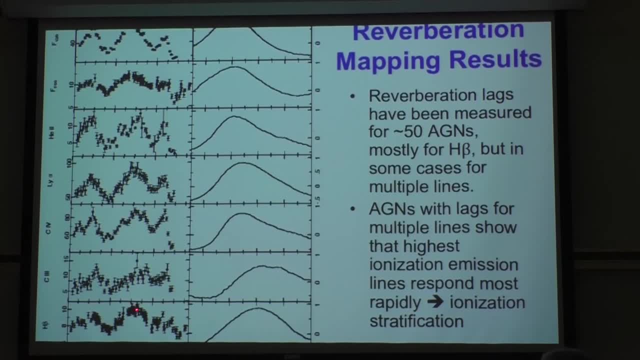 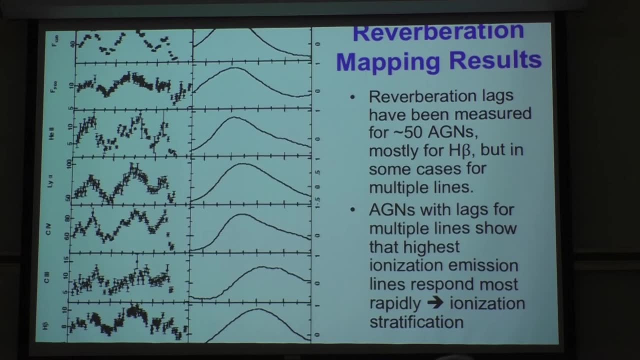 carbon-3, 1909, and H-beta-Bohmer line, Again this one obtained from the ground. And what we see by doing this cross-correlation is that the highest ionization lines, or those characteristic of high ionization media, 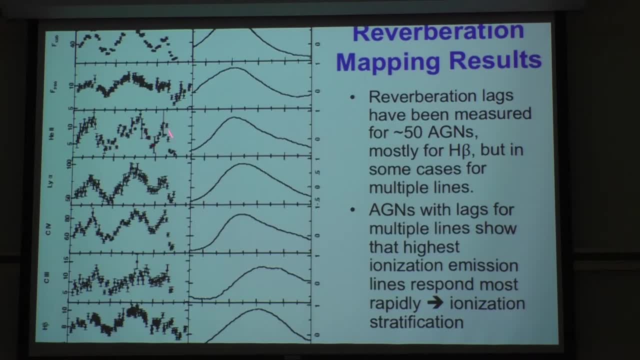 vary the most rapidly and have shorter time delays than the low ionization lines. So we see that the broad-line region, this region of gas that's producing the emission lines, that's absorbing the ionizing continuum radiation from the accretion disk. 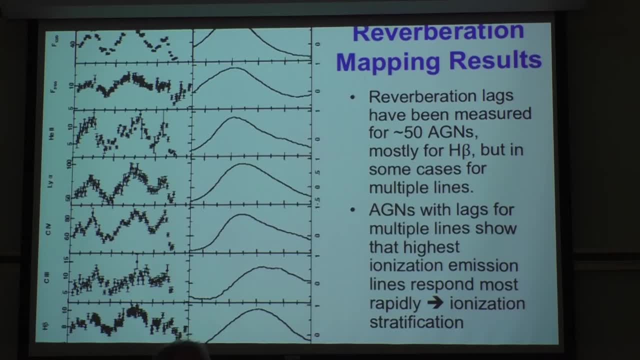 reprocesses into emission lines, We see that there is ionization stratification. in this broad-line region, The highest ionization lines are the closest in which, of course, is no surprise, but it's nice to actually see that physics works. 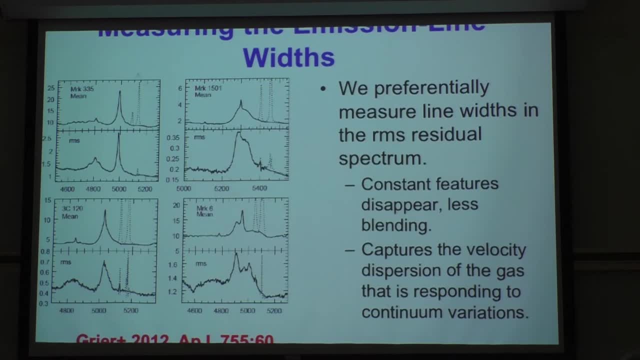 Okay, so when we take these spectra to measure the continuum emission line brightness as a function of time, we can actually take all of these and we can add them all up and we get a beautiful mean spectrum. Now, the other thing that we can do, 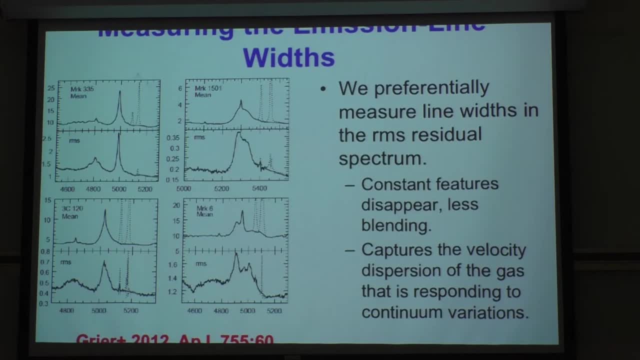 is. we note that they're changing a little bit, you know, from one observation to the next. so we can also take our data and compute an RMS residual spectrum and that isolates the part of the spectrum that is actually varying. So here we see some examples. 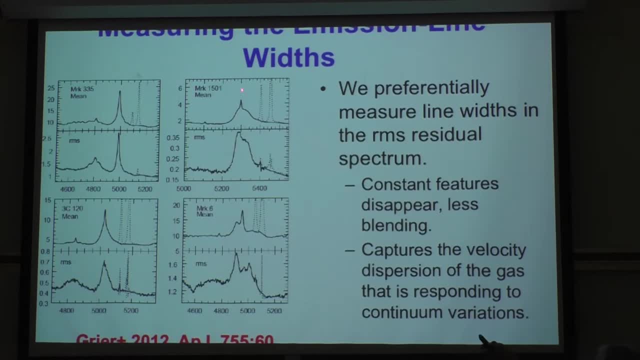 Up on top you see these nice mean spectra that were taken by summing together about 30 to 50 individual spectra, And then below them you see the root mean square spectrum, which isolates the part of the spectrum that's actually varying. 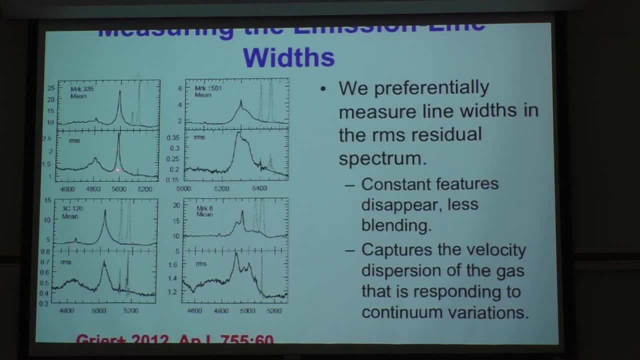 And here, for example, you see nice clean H-beta, the Balmer line and helium-2-4686.. Here again, here you see this very broad H-beta, no helium, for some reason. And then you sometimes, sometimes things get kind of complex, like here: 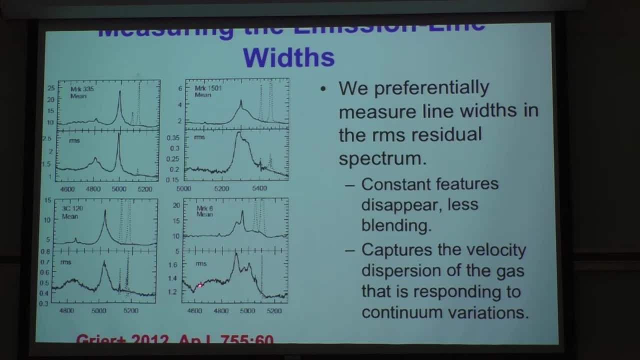 I'm not exactly sure what's going on here, but we've got a blend of helium-2 and H-beta, So this one. this is just to show you that sometimes still, things remain quite problematic, although most of the time we see things pretty cleanly. 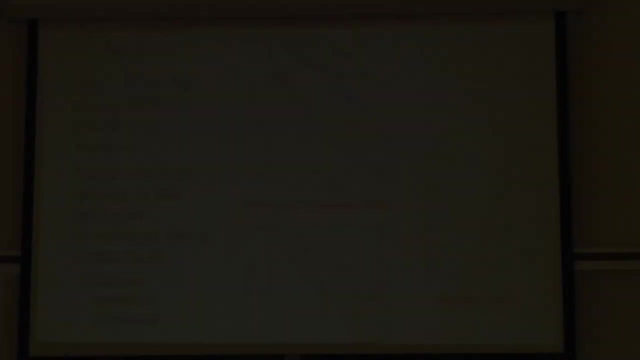 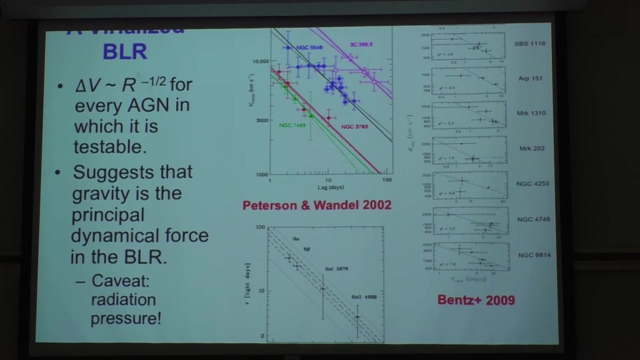 and we can measure the widths of these emission lines. Okay, so now, if we plot the width of each emission line as a function of its time lag, its time delay, we find this extraordinary thing that the line width is proportional to the inverse square root of the size of the region. 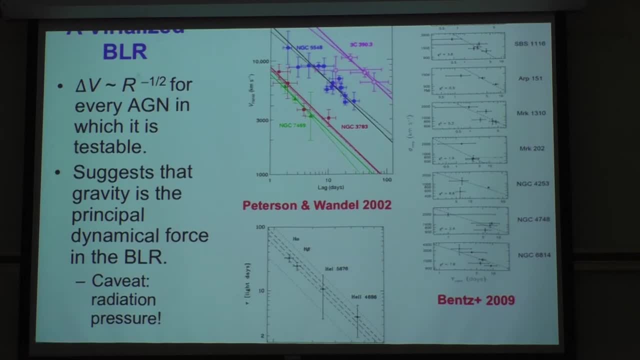 indicating that the product of the line width squared times the time delay is constant. And since the time delay is measuring a distance, essentially what we have found is something that looks like a virial relationship. So we see that basically in every AGN in which we've measured multiple lines. 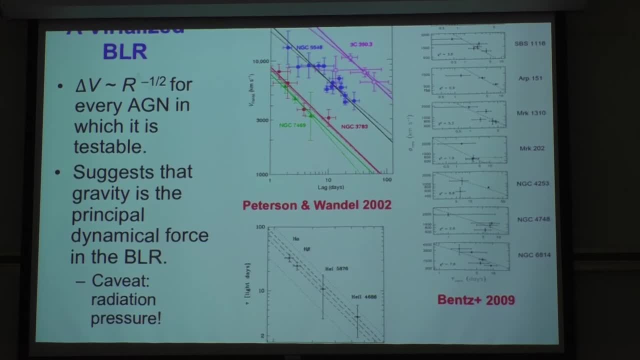 So, again, one of the things we this tells us that the dynamics are being controlled by a 1 over R squared force. But let's also remember radiation pressure is a 1 over R squared force, so we just keep that in the back of our minds. 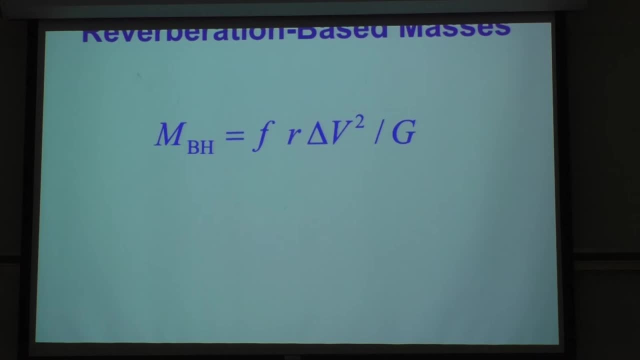 I don't think it's going to be terribly important, but it's one thing you need to keep in your mind. Okay, so now we've taken all these spectra and we've measured two gross quantities, two very simple quantities from the variable spectra. 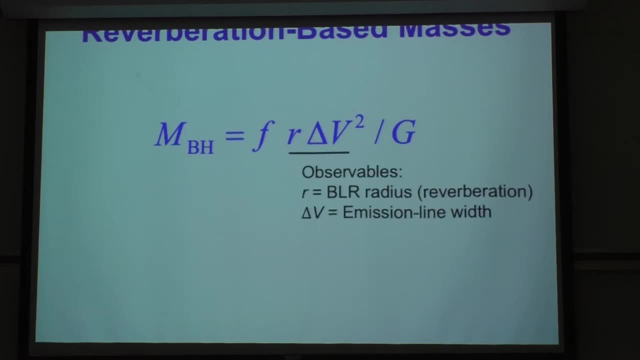 We have determined the size of the region from the reverberation signal and we have determined the emission line width. We can then divide this by the gravitational constant and that puts this into units of mass, But it's still not necessarily the central black hole mass. 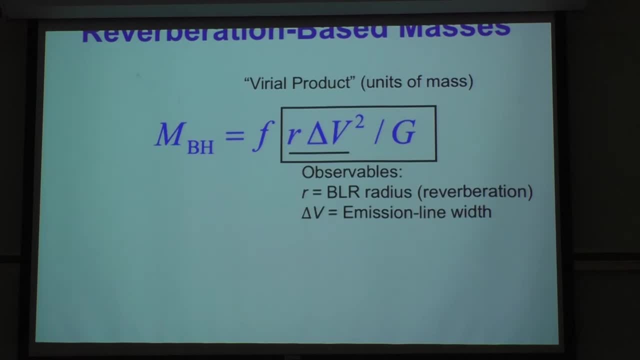 because there's lots of things that we've overlooked in this. Probably the most important- in fact certainly the most important- is what's the inclination of the system. If the system is seen at an inclination of 90 degrees, we're seeing the full orbital velocity of the gas. 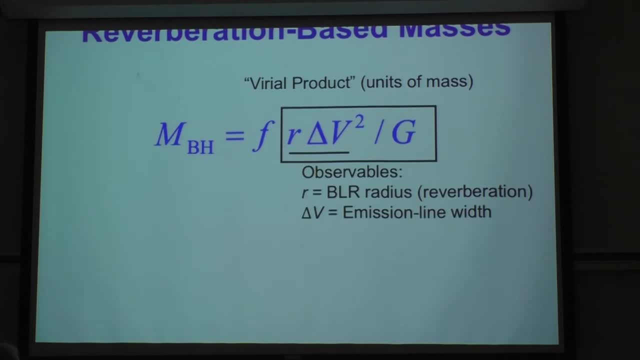 but what if we're seeing it closer to face on? Then we're only seeing a projection of it. So it's going to be lower than we expect And I won't go into it too much. but the types of AGNs that we're looking at 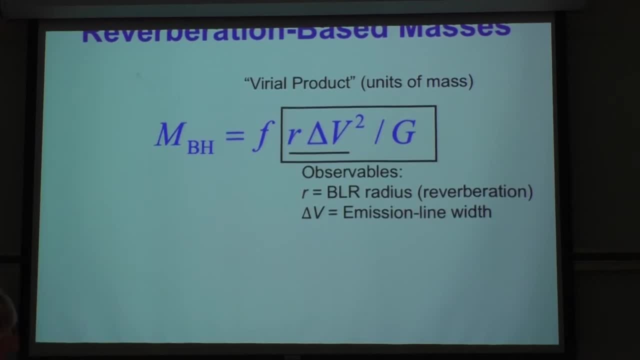 if you can see the broad lines, they're preferentially closer to face on than they are to edge on, So we have to worry about that. So we're going to subsume everything that we don't know into a single scale factor. we'll just call F. 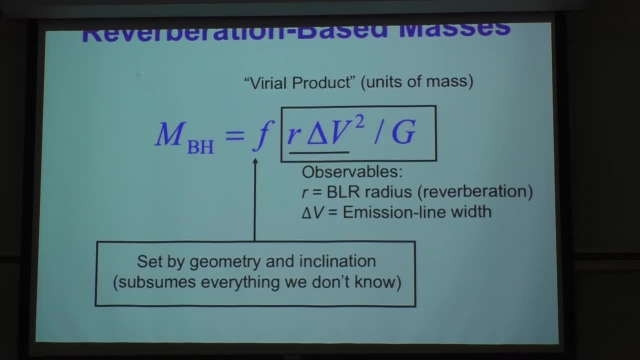 So this is determined by the geometry inclination. Just take everything we don't know and we're going to put it in that number, Because we've got some really crude numbers here. right? This is just the line width and this is the average time delay. 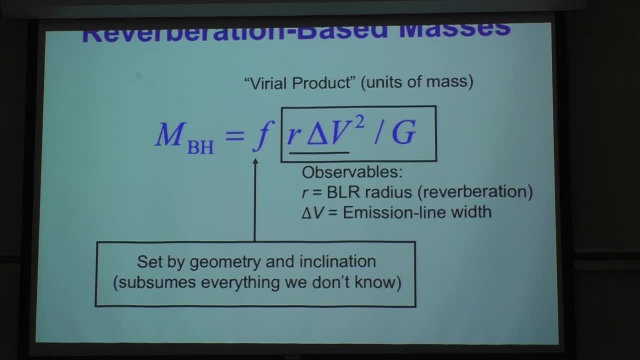 So we're not doing anything very sophisticated here, But oddly we're getting something that seems to be proportional to the mass. Assume that the clouds are going around in circular motion. Not necessarily. That's one of the things we're hiding, this F factor. 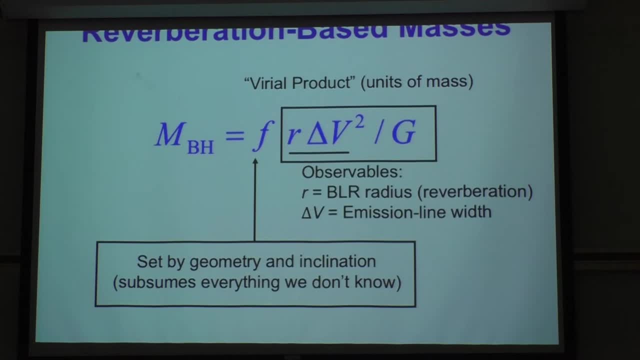 We could look at the recombination lines and see they're not symmetric. I think so they can't become No well, it's complicated. They're optical depth effects. It's not infall or outflow that's making them. 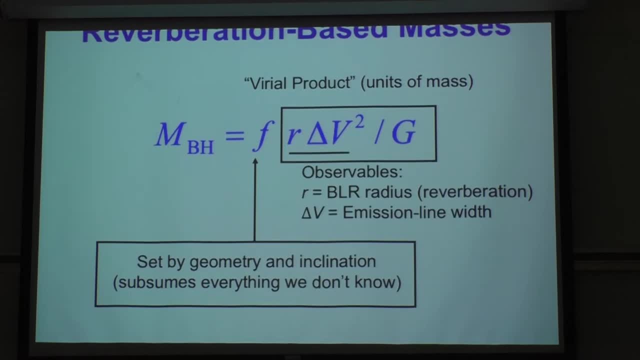 We'll get to that. I mean, right now we're just getting the mass part and then we're going to say, well, we can do better than this. We think we can do better than this, All right, so again. 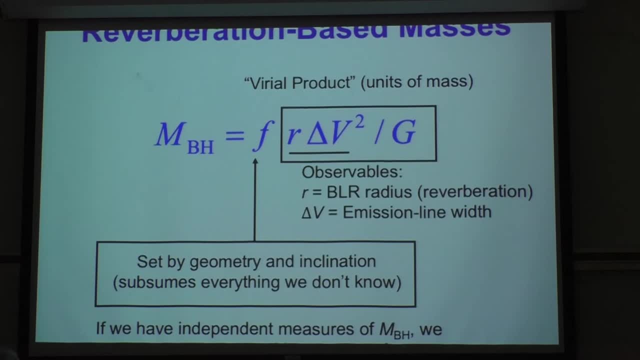 this is partly missing on the slide here, but if we have something else that gives us sort of what an average mass is, it doesn't have to be something that's terribly accurate because we don't have anything that's terribly accurate prior to this. 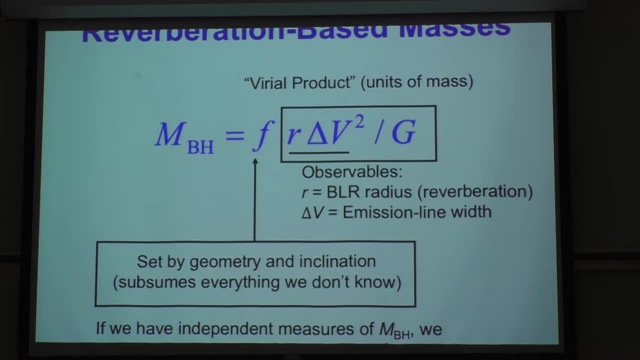 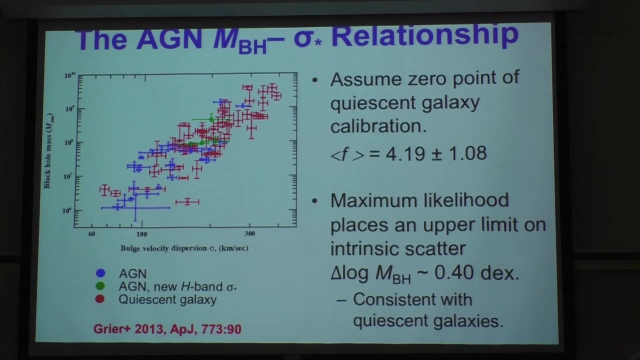 We can compute an average value for this projection factor. So the important thing is we'll get the average population scaled correctly, but any individual mass might be off by quite a bit. So what we use is the relationship between black hole mass and the velocity dispersion of the stars. 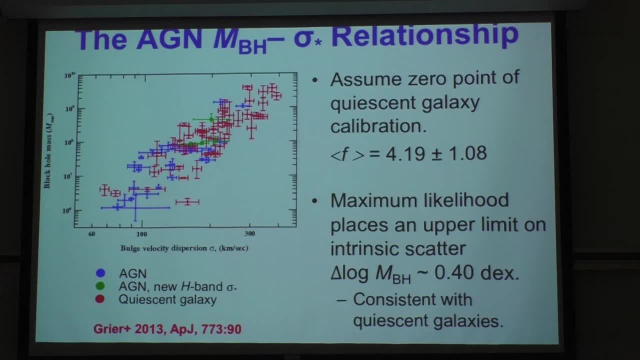 in the core of the galaxy, in the central bulge. So this has been done for quiescent galaxies, those that don't have active black holes, but have black holes. They're just not accreting at high rates In those galaxies. it's pretty easy to look. 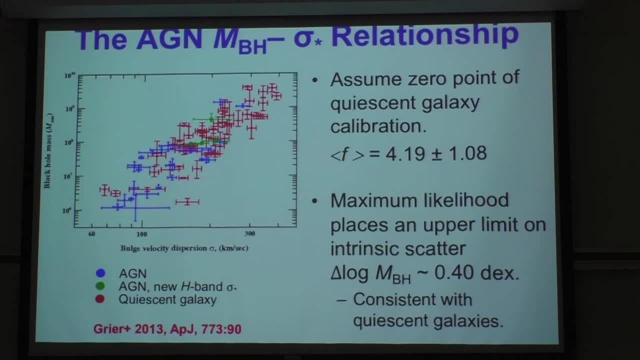 I don't want to say pretty easy, I want to say relatively easy- to look at the kinematics of stars in the core or gas in the core And by modeling that you can get the mass and you can see that there is a relationship. 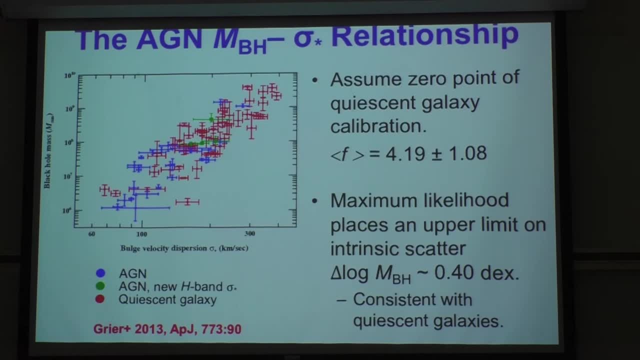 between that and the velocity dispersion of the stars in the host galaxy. It's a very tight relationship, in fact. Now, if we plot on a similar diagram this virial product as a function of the bulge velocity dispersion that we measure in the AGNs, 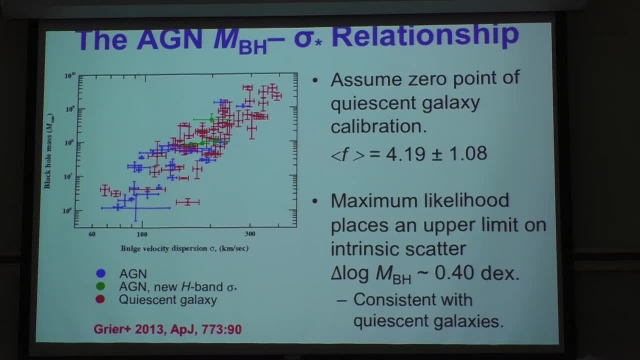 we find that the relationship has the same slope, but it's a little bit lower. So not that it's a little bit lower. that's our average scale, factor F. So what we find is to make these things have not only. 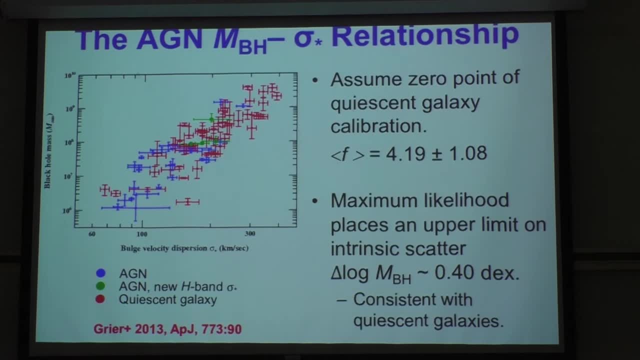 well, they already have the same slope, but to have the same zero point, the F factor has to be something around 4. And that makes these two mass scales then compatible. There are a very limited number of cases where we can make direct comparisons. 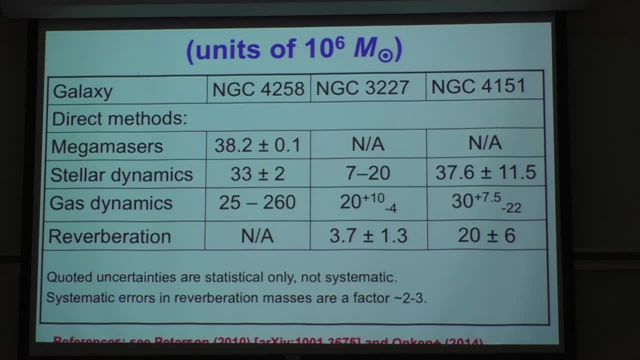 It's simply because to measure the black hole mass using things like stellar dynamics, you have to be able to resolve the radius of influence of the black hole, which means that you can only do this in the very nearest AGNs And we find at the level of accuracy. 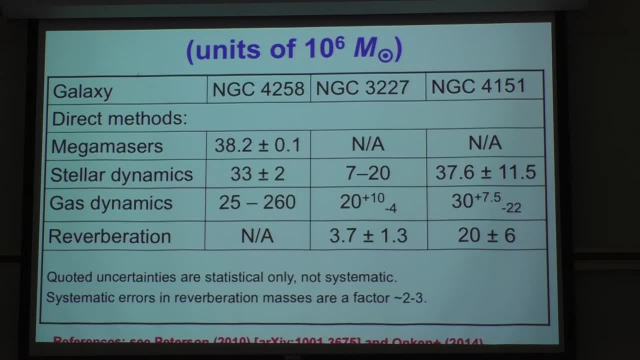 that we can attain right now. they're reasonable. They're in the same ballpark. Okay, now we go out and do this for a bunch of AGNs. We find that there is a relationship between the time lag for any given emission line. 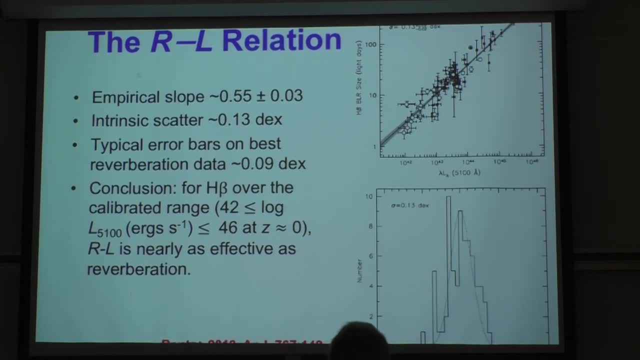 and this is best characterized by H beta. so I'm going to use that. If we look at the time lag for H beta as a function of the AGN luminosity, we see that there's a very tight relationship between them And the slope, the empirical slope. 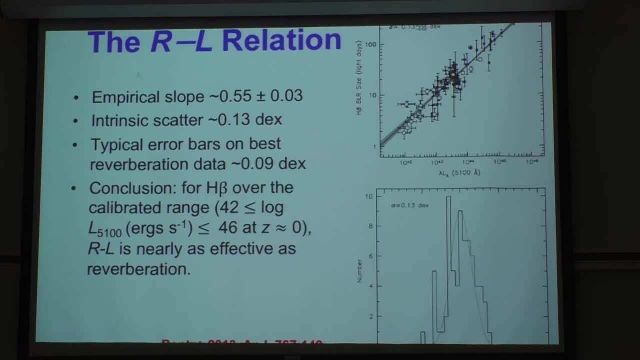 is close to what's kind of expected from simple photoionization, which would be a half. The intrinsic scatter in this relationship is very small, It's about 0.13 dex and that's almost as good as the scatter just from a reverberation measurement itself. 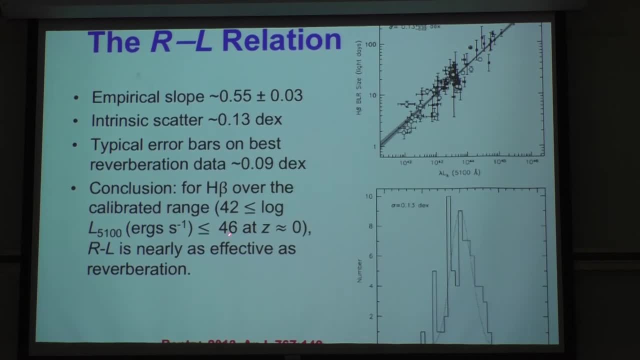 So, over the range that this is calculating, which is calibrated, which is from 10 to the 42 to 10 to 46 ergs per second, you could use this radius-luminosity relationship to get the black hole mass with almost the same accuracy. 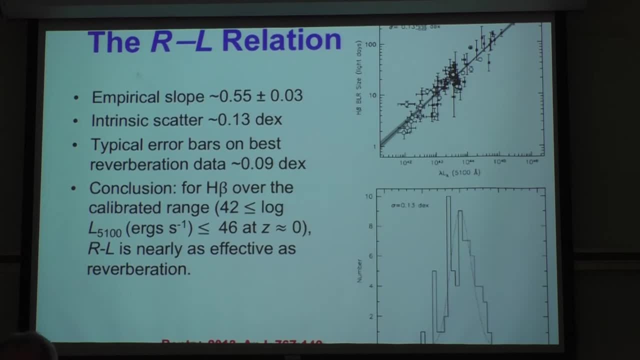 you get from reverberation itself, So you can do this with one spectrum instead of 30 to 50 spectra. You need 30 to 50 spectra to get a good reverberation result, but with one spectrum you can measure the luminosity. 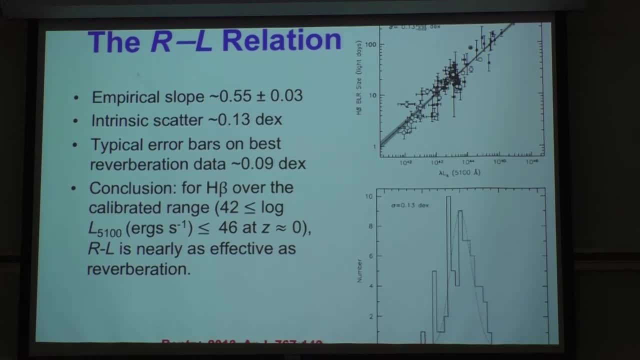 you can read off this diagram based on the region. you can combine that with the line width and you've got a mass. So this is how you get the masses to quasars. It all comes back to this. It's all tied to the reverberation masses. 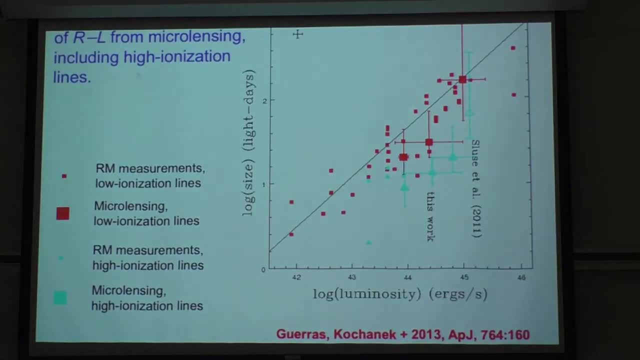 but it's based on these scaling relationships. Okay, the scaling relationships are also seen in gravitational microlensing, And what happens with this is that if you're looking at a lensed source, a quasar, that's lensed by a galaxy in between us and it 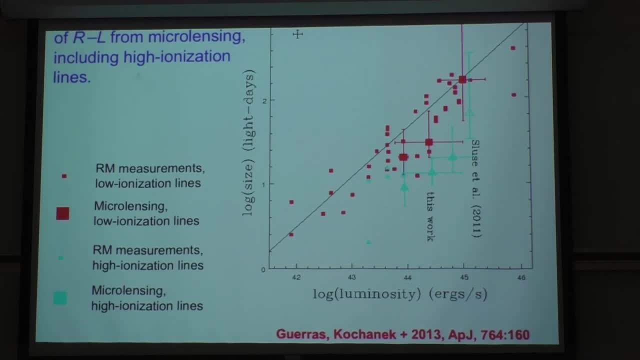 as individual stars move across the AGN nucleus, you see small variations And by looking at how wide those variations are, it gives you an idea of the relative size. So what you find using gravitational microlensing is you see the same relationship between the size of the emission line region. 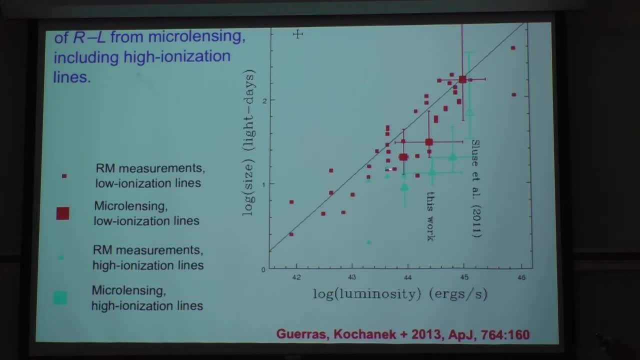 and the luminosity of the AGN. Now, the big symbols, of course, are microlensing. You can tell that this is a microlensing slide, It's not mine. And there's two ways you can tell. One is: the microlensing symbols are the big ones. 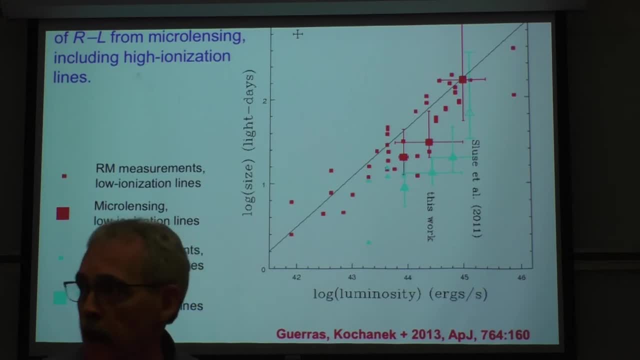 and the other is they are plotting cyan on a white background and don't ever do that, So okay. so this is- Let's look at the red symbols here- This one's spot on. These are a little bit displaced, but they're displaced to the right. 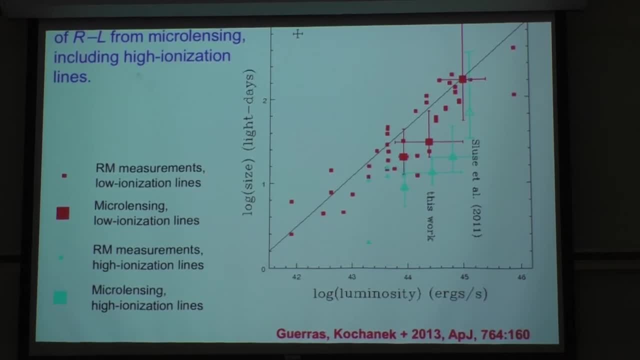 because the contribution of the host galaxies of the starlight has not been removed and that would move these over here. So all of the AGN reverberation results we have taken out of the measurement, the host galaxy starlight contribution And in cyan you can barely see here. 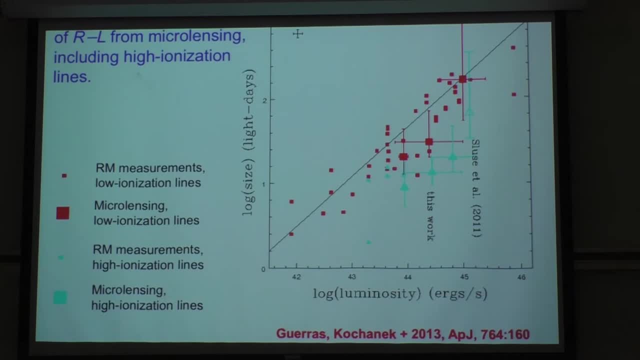 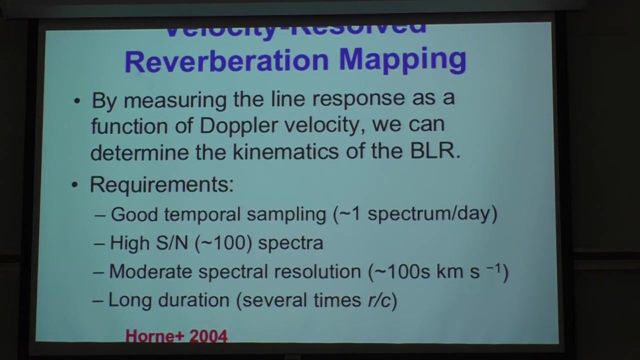 this is also displaced, but these are higher ionization lines. The higher ionization lines, then, are closer to the continuum source. So you're seeing again ionization stratification. So there's independent evidence that this actually works. Again, I'm sorry. 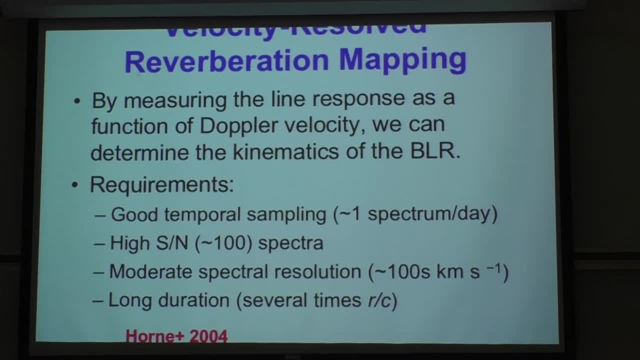 I don't have the slide here, but Oh yes, all right, All right, Cool, All right, I'll just continue Now. there's a bunch of information that's available in these spectra that we haven't made use of. 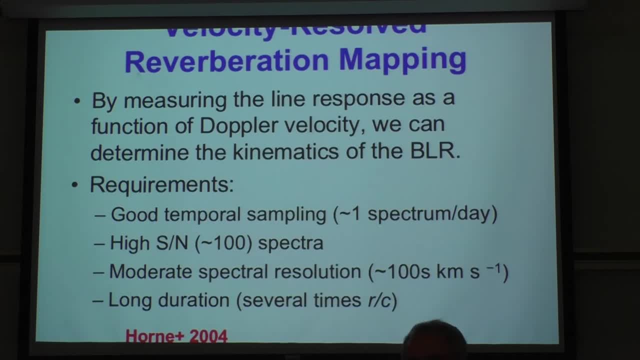 and specifically that we should be able to carve up the emission line into velocity bins and see how each individual velocity bin responds with time. We've started to realize that we could do this. about 20 years ago and Keith Horn and some others and I got together and said: 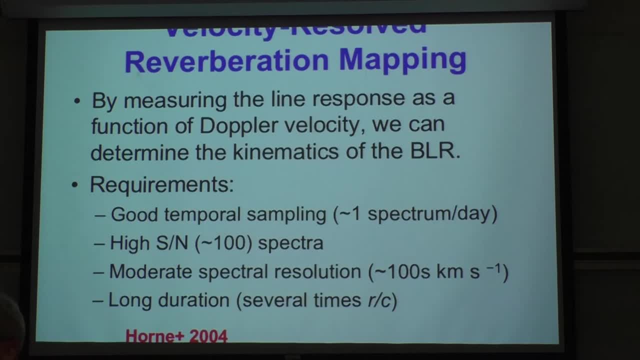 all right, let's do some simulations to figure out what would it take to actually really recover, what the time and velocity dependent response looks like. And the requirements are pretty high, but they're not daunting. You have to get basically for relatively nearby AGNs. 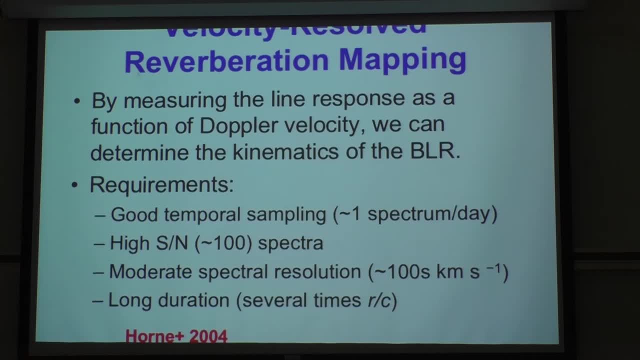 you have to get one spectrum a day. No more of this once-a-week stuff. You're going to have to go get it every day. The spectra themselves have to be high. signal-to-noise Spectral resolution doesn't have to be extraordinarily high. 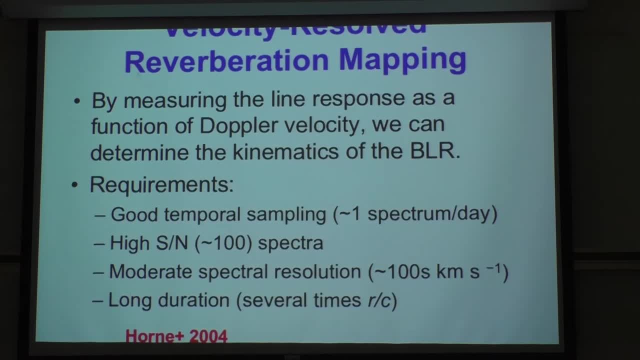 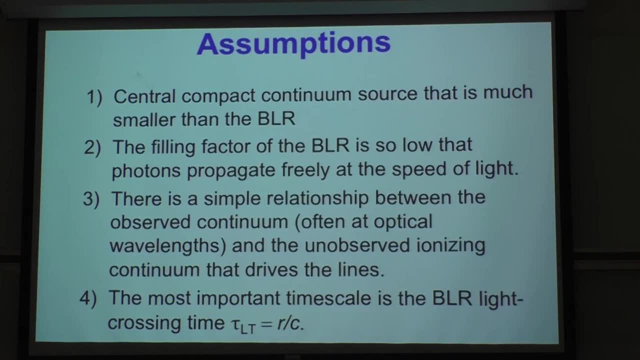 And the experiment itself is going to have to run for quite a long time. So we run these things for months, typically observing every day. Now we make some simplifying assumptions to see how this works. We're going to assume that the accretion disk 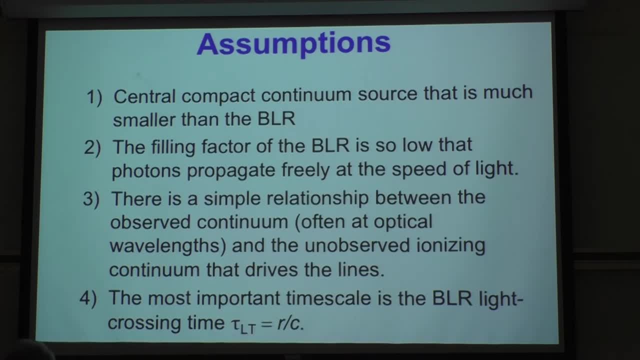 is very small compared to the line emitting region. It is very small. It's essentially treated as a point source. We're also going to assume as a starting point that the region is made up of a bunch of individual clouds and the filling factor is quite small. 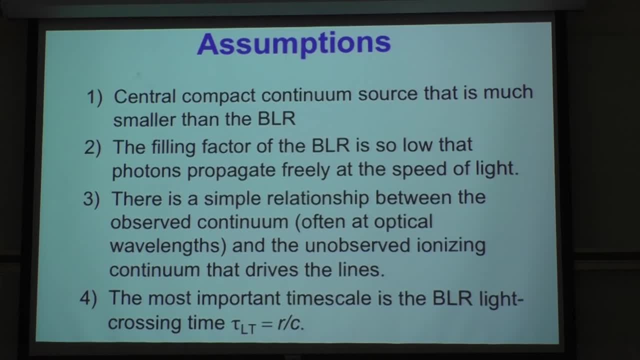 So when they convert an ionizing photon into an emission line photon, it can freely escape from the region. We'll also assume that the continuum that we can observe, which is the optical or satellite ultraviolet continuum- we're going to assume that that serves as a proxy. 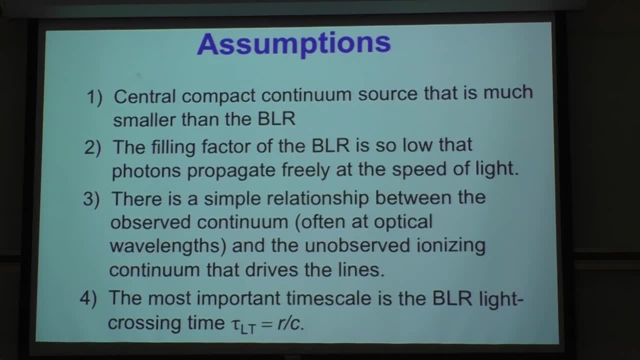 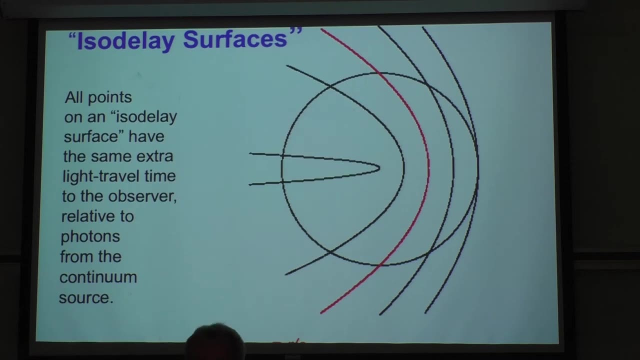 for what the ionizing continuum is doing, And we're also going to assume that the most important time scale that we have to deal with is the light crossing time across the broad line region. Okay, so the basic idea is: let's see if we are sitting at the center of an AGN. 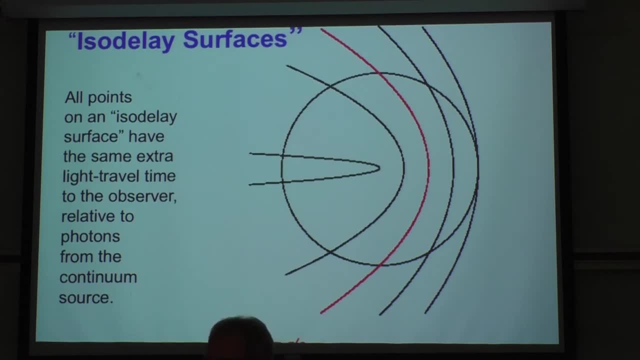 and we send a flash. a big ultraviolet flash bulb goes out spherically and hits the clouds. clouds turn it back into ionizing radiation and some of it comes back towards us And we would see like 10% of the sky. 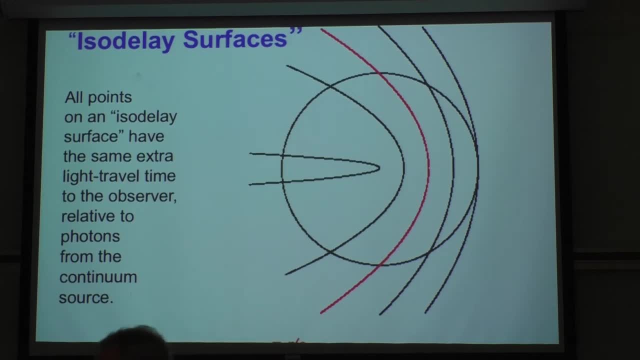 which is sort of the covering factor of the clouds. we'd see 10% of the sky simultaneously flash back at us at a time delay, two times the radius divided by C. One ROC going out, one going back- We see the whole sky flash at once. 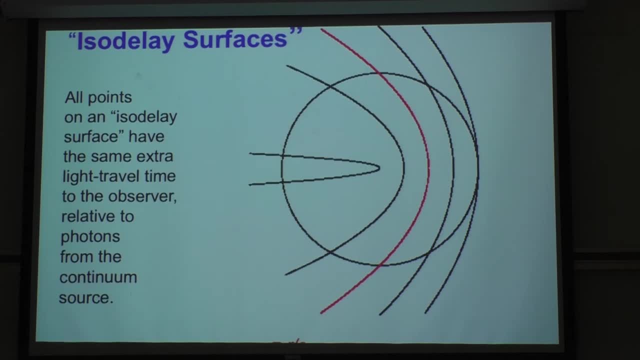 because we're at a privileged location. If we're anywhere else, we'll see different parts of the region respond at different times And the locus of points that you're seeing respond at any time to this outward flash is going to be defined as an isodelay surface. 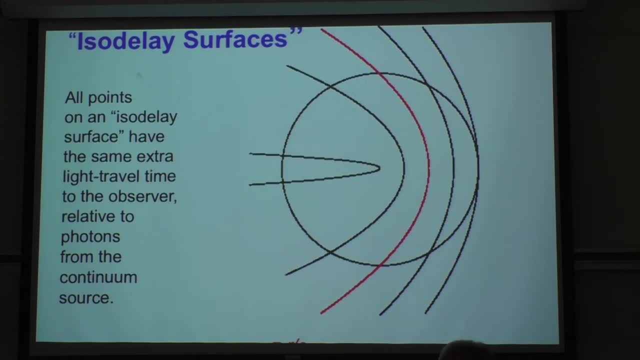 and you know what happens when you have a locus that has one point, the distance from one point to the locus, to the observer, to the other point, that's an ellipse right. And if you take the observer and move them to infinity, 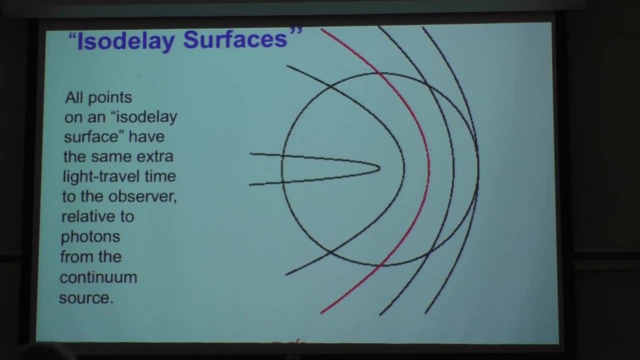 it becomes a parabola. So what you're going to see is, initially, the response material is going to be, that's along the line of sight, and then the response of nested parabolas as a function of time. So at any given time, 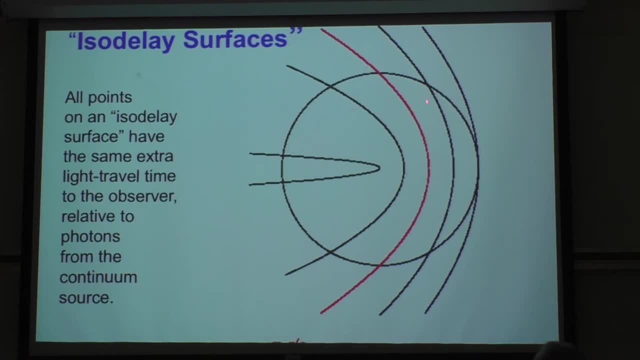 the material that you see responding is going to be whatever line-emitting material is on this particular isodelay surface. So you can see that the time delay relative to the continuum photons which just head off in this direction for this particular surface is ROC. 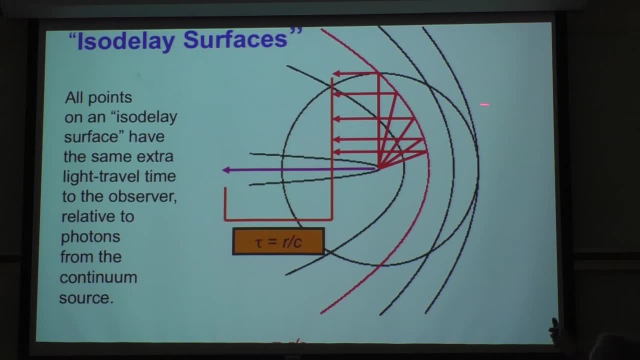 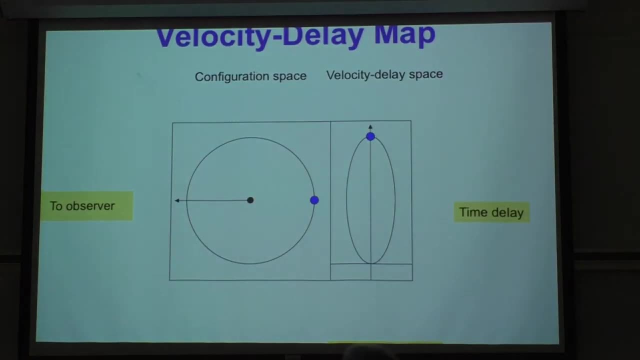 So the points that we'd actually see responding if we had a circular broadline region, clouds on a circular orbit, would be the points here and here. Okay, so we can sort of- we'll do a little cartoon version of this, the kind of thing that one would show. 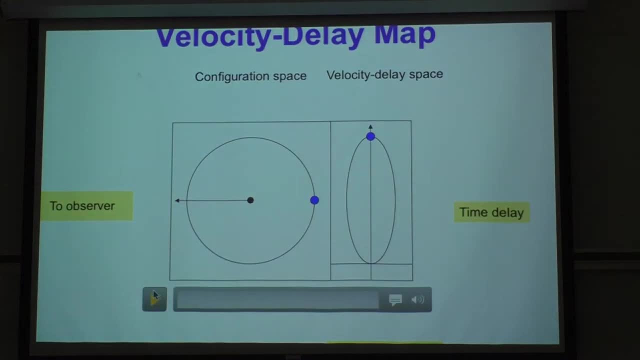 in a freshman physics class. There we go. That, as a cloud circulates, revolves around the black hole in configuration space. we want to put this in terms of our observables, which is time delay and Doppler shift. Those are two observables. 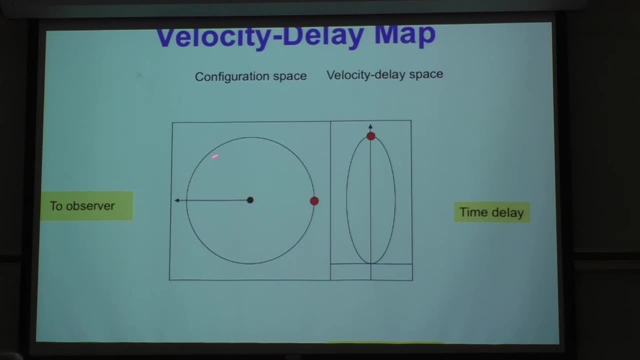 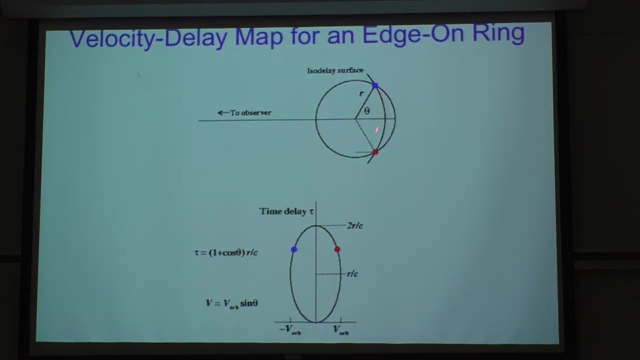 So what we see is that a circular orbit in configuration space translates to an ellipse in velocity time delay space, which is where our observables are Okay and you can see. it's very simple geometry that you have here. We have defined an angle, theta. 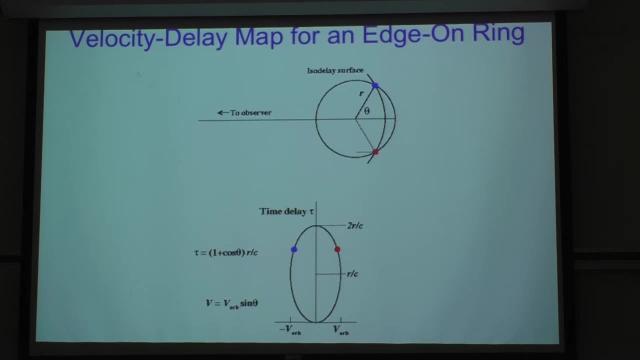 off the axis to the observer. And again we see that points say right along the line of sight, respond instantaneously and the velocity is entirely transverse. So at this point you have zero velocity and zero time delay. At the far end you would have a delay. 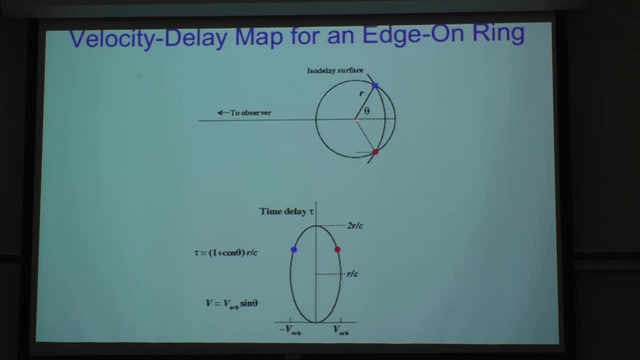 that's two R over C, as the photons go out, get reprocessed and then come back and have to catch up, So that projects to this point. here The highest velocity is going to be right here where it's R over C. 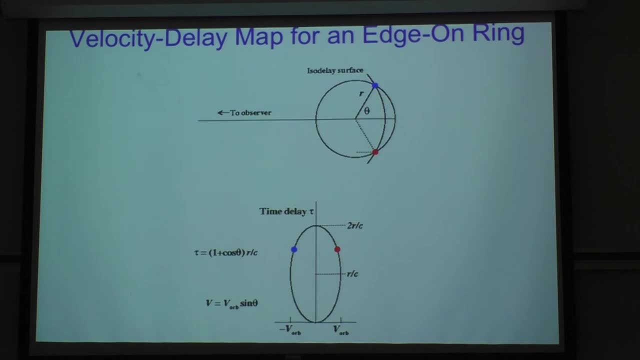 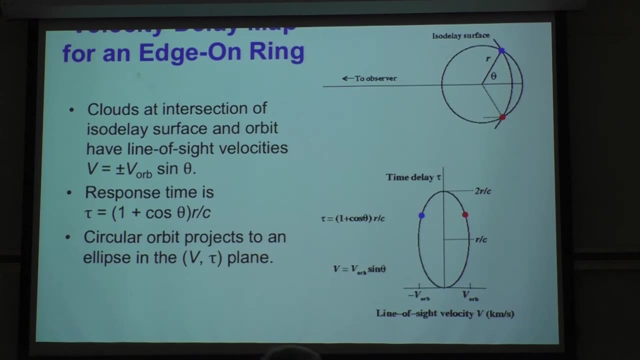 and the entire orbital velocity is along the line of sight. So, again, this is how it projects, And okay. so if we look at the response then of a ring of clouds that we see edge on, it's going to project to a locus. 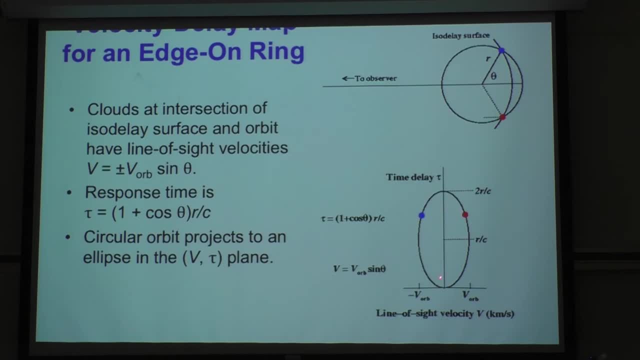 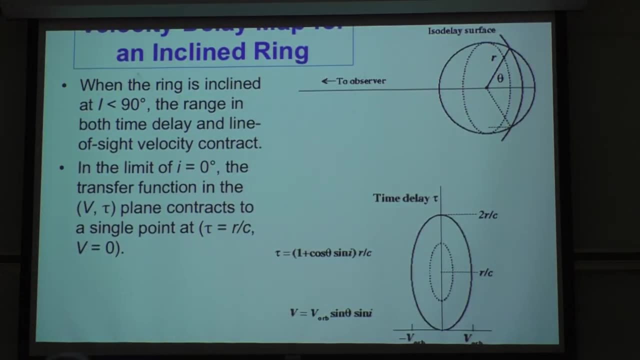 in velocity-time delay. that has dimensions, as you see here, And if we tilt it a little bit, right, if we tilt the ring a little bit, the ellipse begins to contract in both directions. and the extreme case would be if you had a ring that you saw face on. 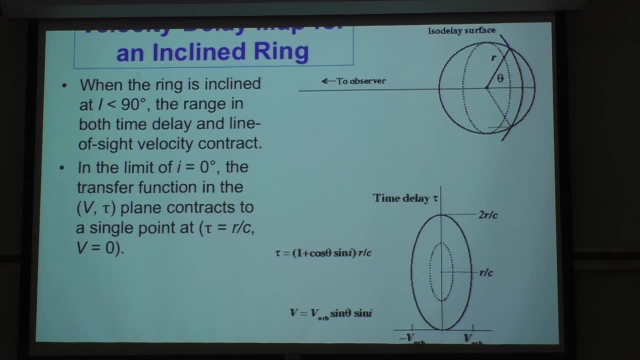 then all the time delays would be identical and the Doppler shifts would all be zero, because the orbital velocity is entirely in the plane of the sky. So an important thing to keep in mind. So this is how inclination will affect our velocity-time-delay map. 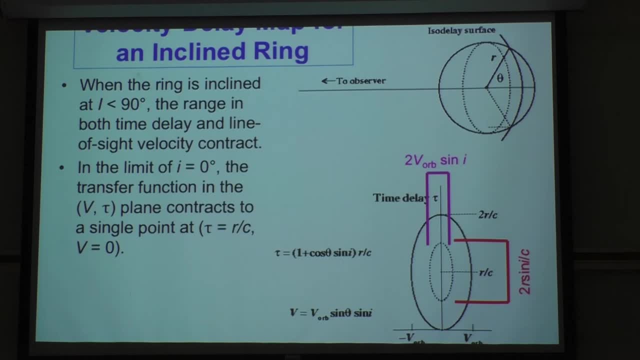 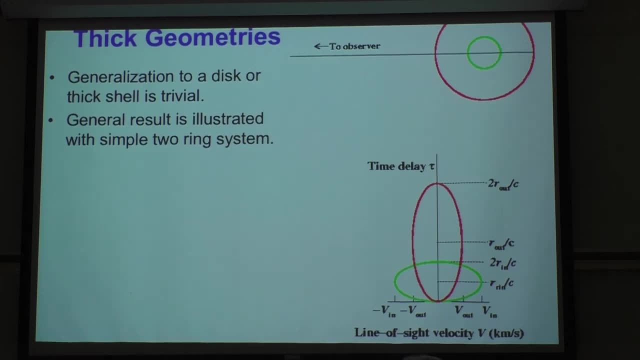 which is what we're constructing here And again it projects in both directions by a factor of sine, of the inclination. Okay, so if I want to go to the thick geometry, something more complicated, I can look at a disk, for example. 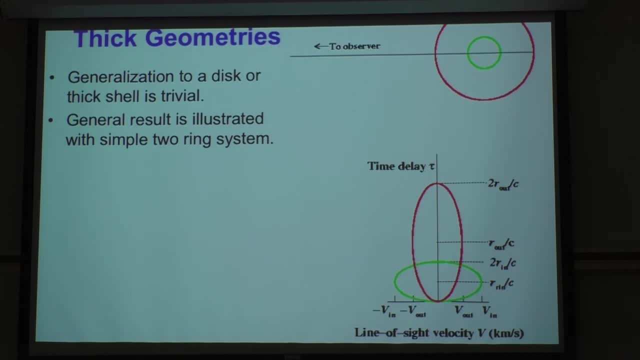 and disks are good things to look at. I can make a disk out of a nested string of rings, and if I bring a disk and make smaller rings, of course they're going to have larger Doppler velocities and smaller time delays, So they also project to an ellipse. 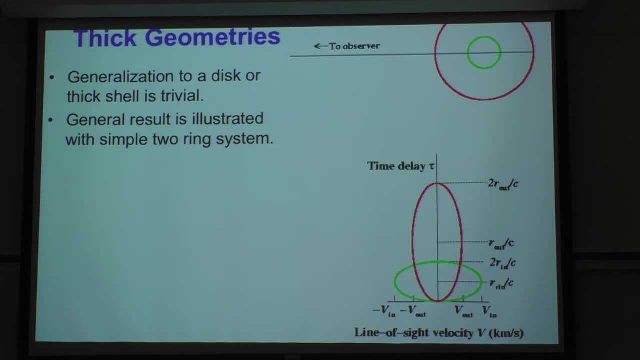 but an ellipse that is shorter and wider, as seen in velocity-time-delay space. If I add up several of these, you can start to see this sort of characteristic response. This is the characteristic response that you would expect for a multiple-ring system, which you can interpret then as a disk. 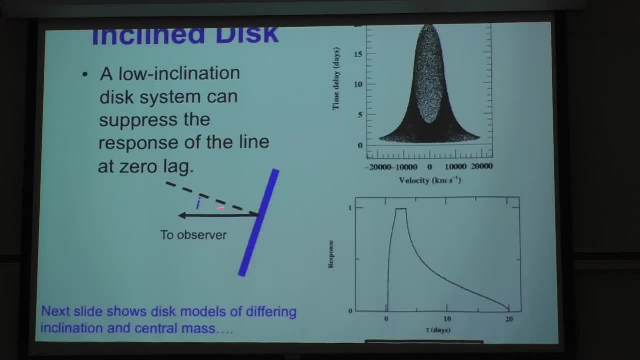 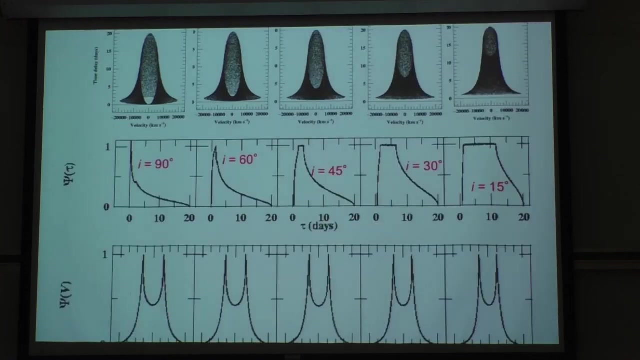 Okay again, if you incline it somewhat, you'll see the same sort of structure, but now there is a gap here that you see between this ellipse and zero time delay, And I'm only bringing this up because inclination will turn out to be important later. 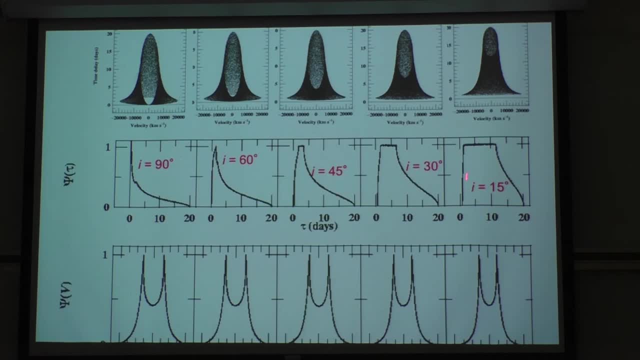 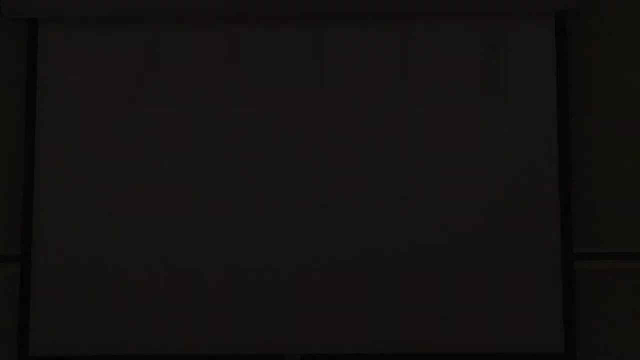 Again, you can see that as you go to higher and higher inclination, this ellipse becomes smaller and smaller and more displaced from the zero time delay axis. Okay, and just to reinforce this yet one more time, we made a little movie here that shows how a flash. 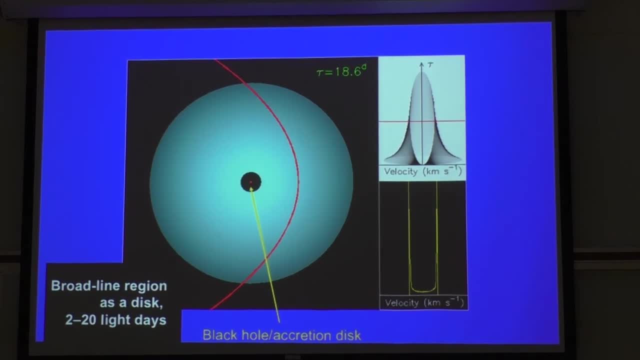 how a flash propagates through the region. This is a particular frame of a movie. So here we are in configuration space with a disk that goes from 2 to 20 light days. This is one frame of the movie where the iso-delay surface is at 18.6 days. 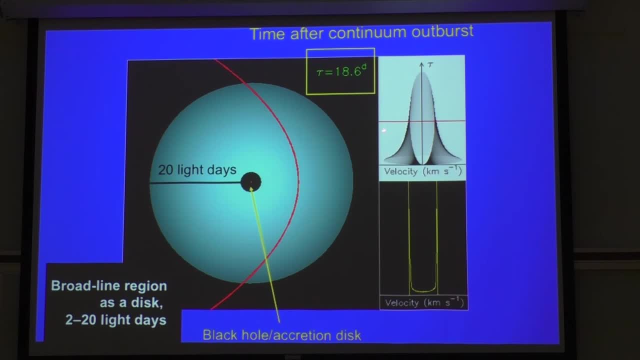 If we look in velocity-time-delay space, we see of course that the surface, that the iso-delay surface, is just a straight line here. And if we look at the intensity of the response across this iso-delay surface, we see the emission line profile. 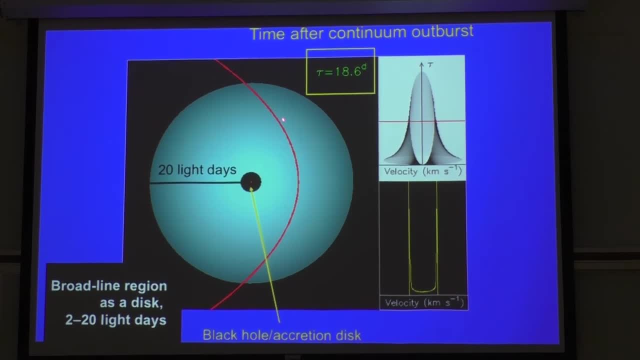 the instantaneous emission line profile. This is the gas that's along this particular delay surface here. This is how it's responding. So and again, we got this time delay and this is in configuration space projects to a line here. So what we'll do is we're going to run the 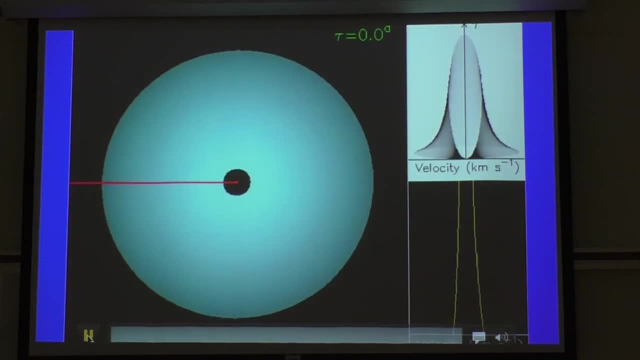 Oh, tragic here. This is how the system will evolve if you set off a flash bulb at the center. This is how the emission line would change with time. So I'm going to run that through one more time, just because it's kind of cool. 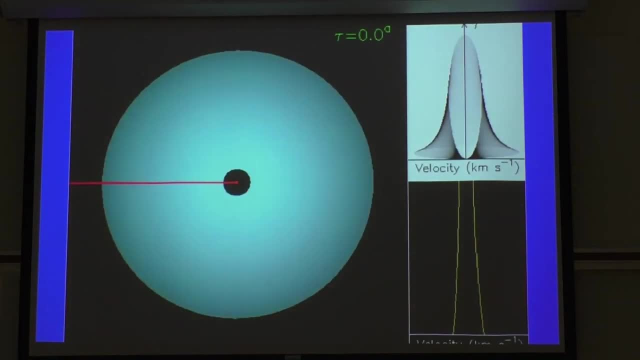 And I hate touchpads, hate them. There we go. Okay, there we go one more time. Okay, this would be really easy to see if AGNs emitted single pulses. right, But they don't. They have this irregularly varying continuum. 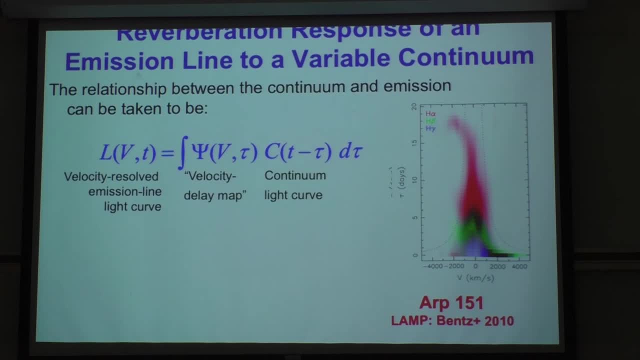 And at any given time, the velocity resolved. The emission line light curve that we're going to see as a function of now line-of-sight velocity and time is going to be given by a convolution of the continuum over its recent history, with the velocity delay map. 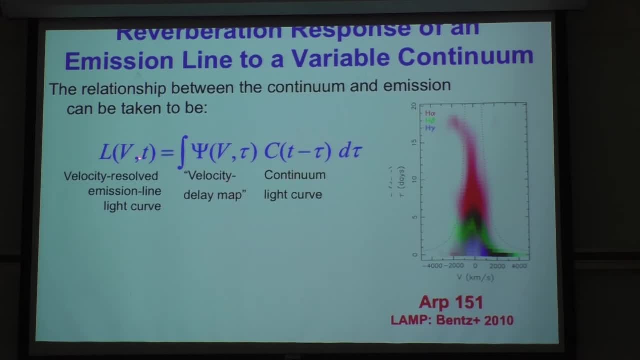 And now, if you imagine that the continuum is a function, then what you see is that the velocity delay map is simply the observed line response to a delta function outburst. So this is what we want to try to recover. This is actually what a real one looks like. 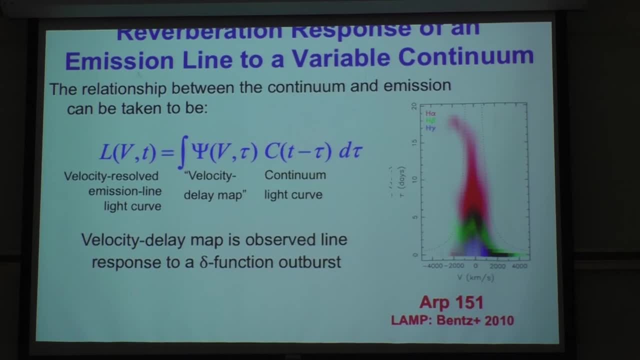 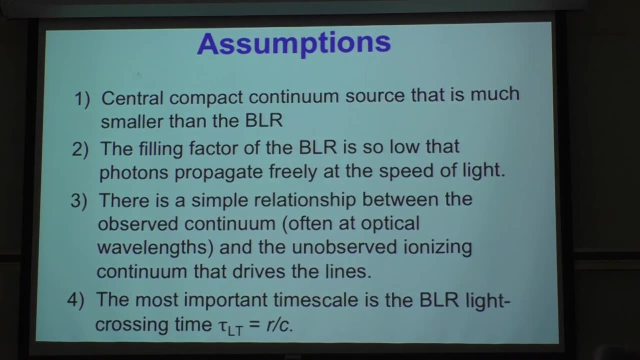 This is a composite of three different emission lines: H-gamma, H-beta, H-alpha- Okay, talk more about that later. So this is hard to do and we haven't done it in a lot of cases And, in fact, these assumptions that we used- 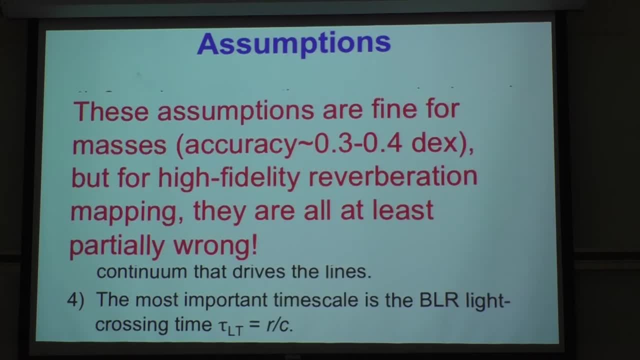 to make this little model about how things work. it turns out these are fine for getting masses, the accuracy of about 0.3 to 0.4 dex. But if you want to really study the dynamics of the gas, what you find is that at some level, 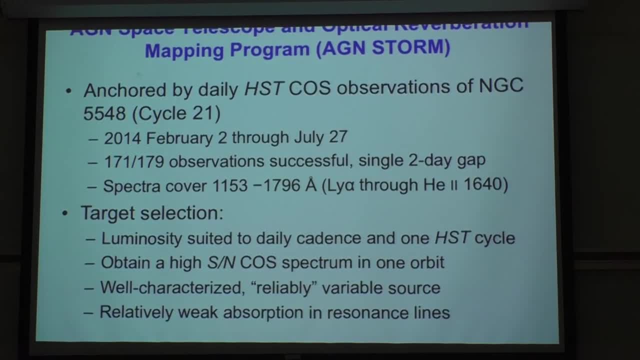 all of these assumptions are wrong. All right. how did we show that? Well, the way to do that is to get better data right, Get data that really challenge the technique. We had a successful Hubble Space Telescope program in Cycle 21,. 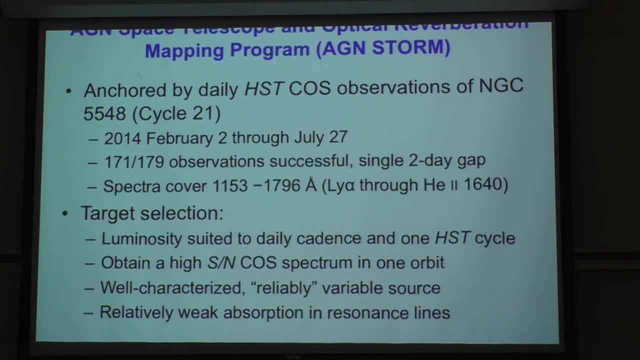 which was executed then in the first half of 2014.. We, for a half a year, we observed in the ultraviolet every day the same AGN and looked how it evolved over time. The target that we selected was one that was suitable for daily sampling. 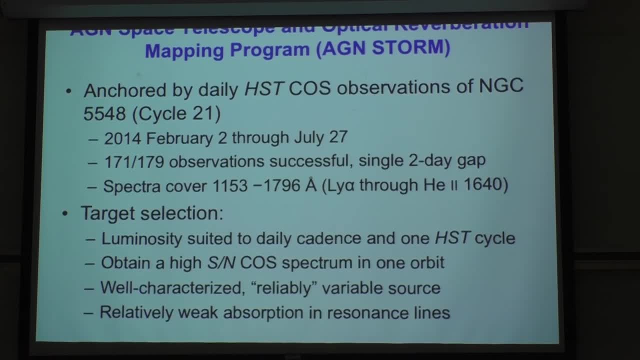 that you could get a cosmic origin spectrograph spectrum of it in one single orbit And it's a source that we regarded as reliably variable And the absorption lines in the ultraviolet were relatively weak because the strong ultraviolet lines are all resonance lines. 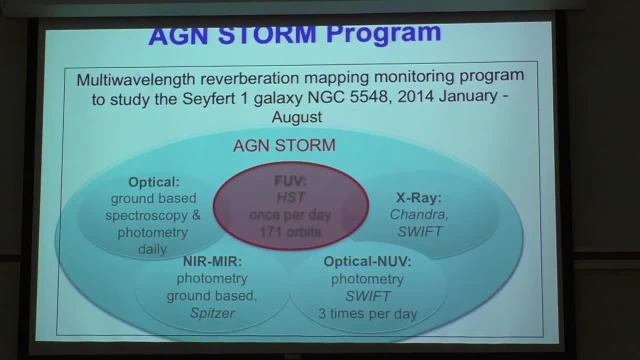 so they're subject to self-absorption different than H-beta. Okay, so around this we built up additional observations with ground-based telescopes and other space-based telescopes, including SWIFT, And fundamentally we've had some surprises. We see that there here. 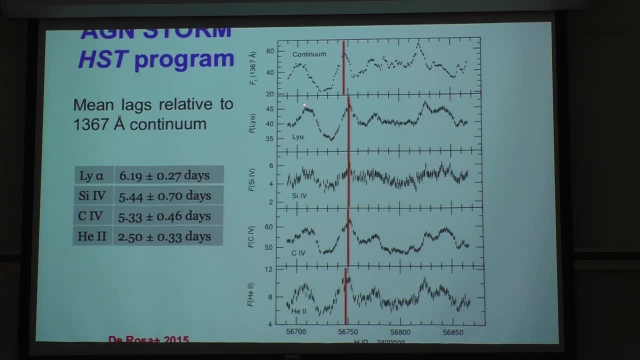 are the variations that we see in the continuum. This is what we see in Lyman-alpha, silicon-4,, carbon-4, helium-2, 1640.. What you find we did not see the same ionization stratification that we saw in the same object years earlier. 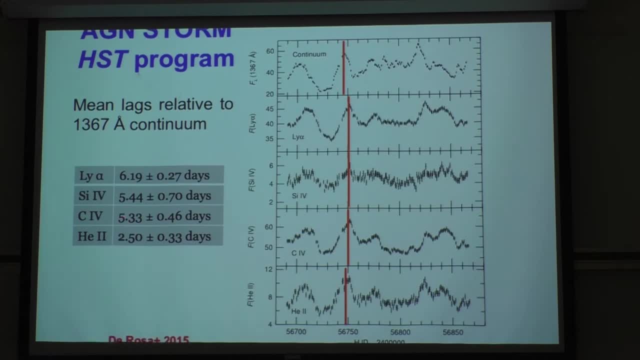 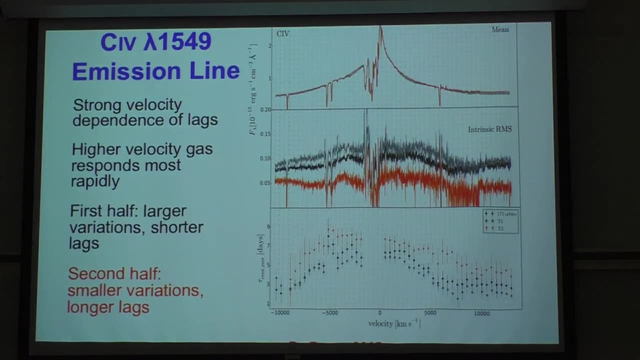 We see that helium-2 responds a little faster, but the response of these other lines is basically indistinguishable. They're all about the same: The. we also found that the, the emission lines- this is carbon-4, are tremendously eaten up. 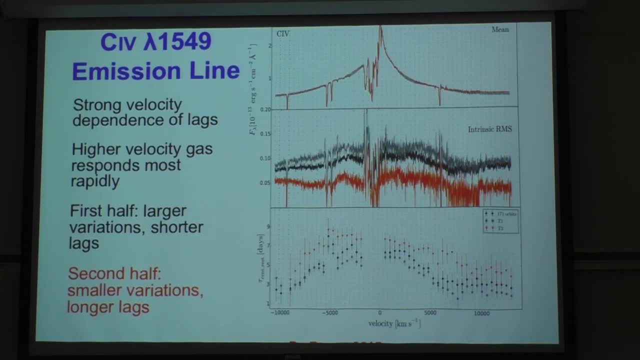 by both strong and narrow absorption features And when we try to look at the average lag. this is a crude way of doing this. we just take the light curve in each velocity bin, cross-correlate it with a continuum and we get some kind of a measure of the time delay. 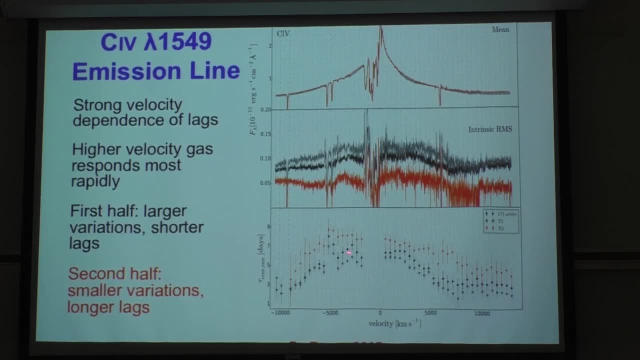 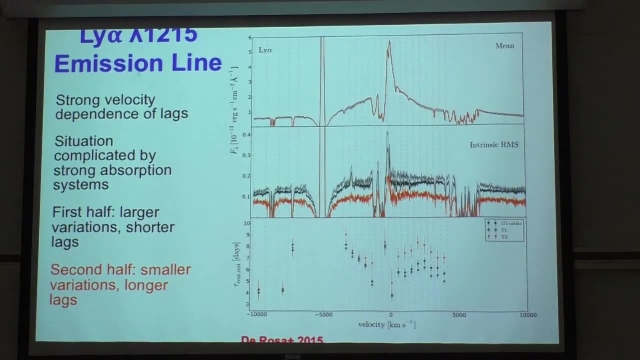 So this kind of fits our intuition that the slowest moving material is the farthest away from the black hole. but the pattern is not really recognizable. Lyman-alpha has a lot of problems, not only the absorption that occurs in the vicinity of the galaxy. 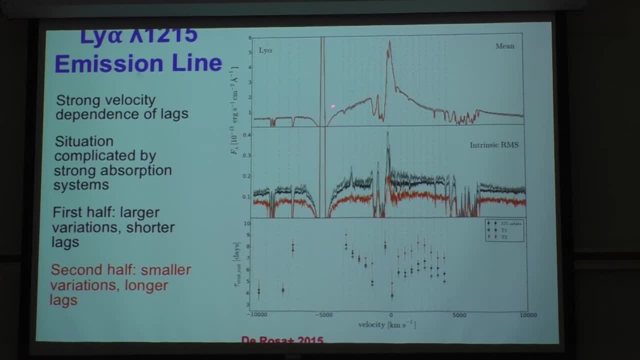 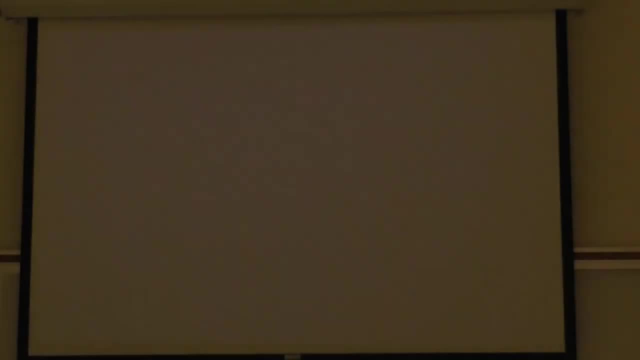 but here's absorption that occurs due to our own galaxy and superposed on top of that is strong emission due to Lyman-alpha geocoronal from the Earth's upper atmosphere. Oh, wrong button. okay, H-beta not subject to absorption. 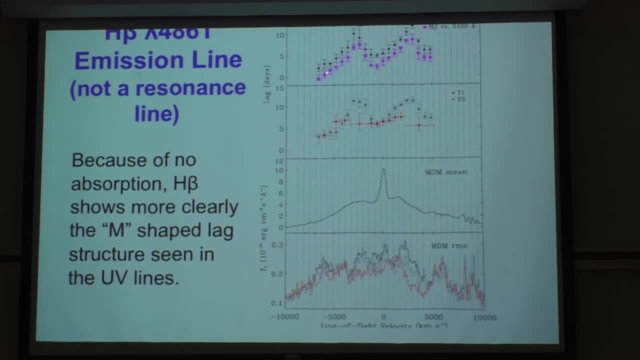 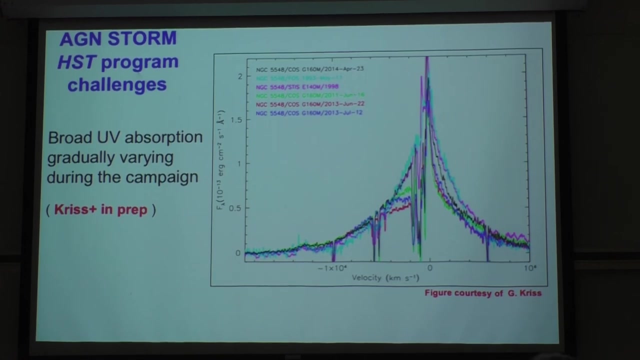 but still shows an interesting pattern of velocity response. We're seeing that the lowest velocities, which we expect to have the largest time delays, actually don't. We can explain this and we'll get to it later. All right, so the absorption posed a real problem for us. 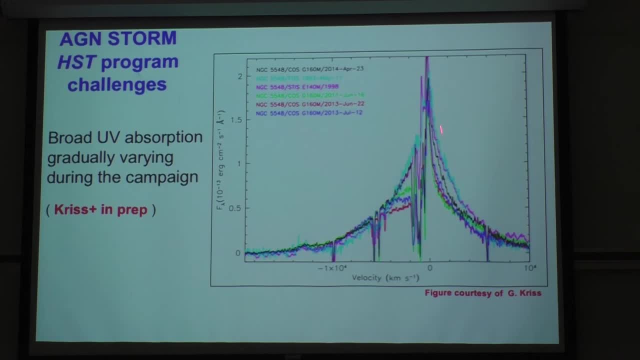 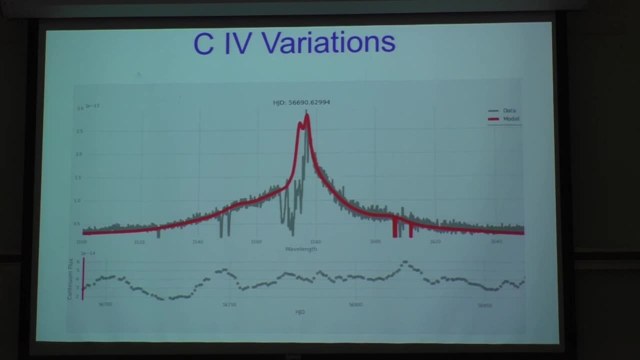 What we had to do is we had to look at historical spectra where there was less absorption and try to model each individual HST spectrum to eliminate effective absorption so that we could just study the emission line variations. This was not easy because we had to develop all this software from scratch. 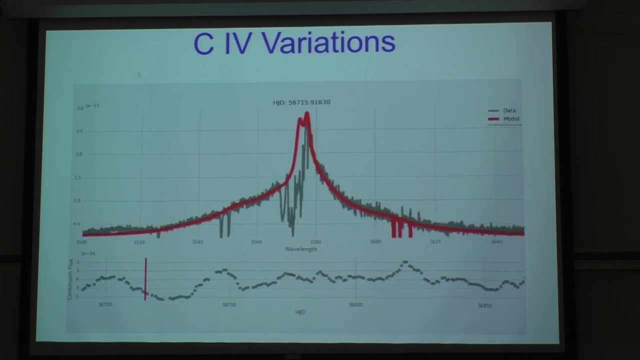 and this basically represents the work of two people here, which is why I'm showing you every one of these spectra. So what we're going to be doing, instead of actually modeling the data, we're going to be modeling the model data because we have to take out the effect of the absorption. 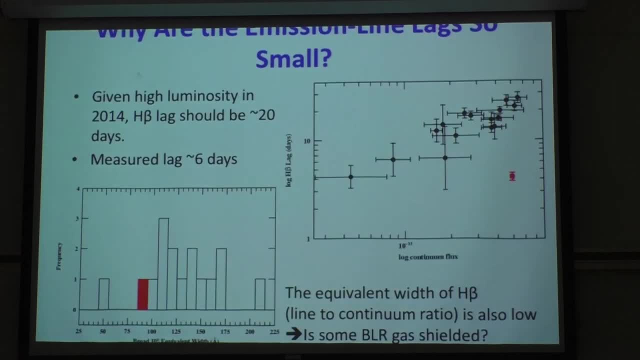 Actually, you've probably seen enough, so we'll move on. Okay, another thing that we need to consider mostly. we've observed this source many, many times. Almost every year we have a reverberation campaign on it, and over time. 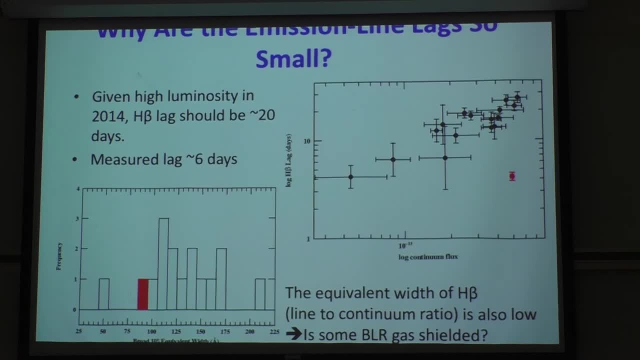 we see that the emission line time delay for each beta can vary from as short as a few days to as long as 20 to 30 days. Yeah, this is 30 days up here. We would have known if we'd only had optical data in this campaign. 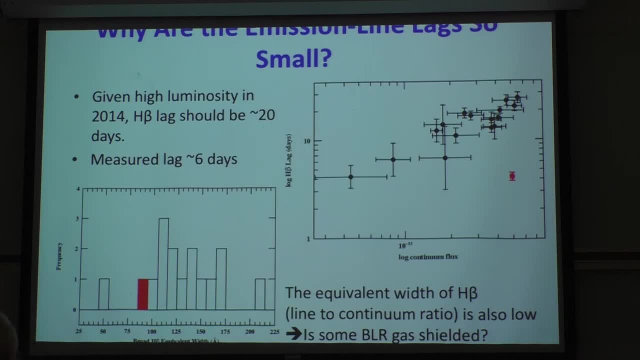 we would have known something went weird And the reason that we would know that is, first of all, the equivalent width of the emission line, which measures the emission line strength compared to the continuum underneath. it was very low For the amount of continuum they were getting. 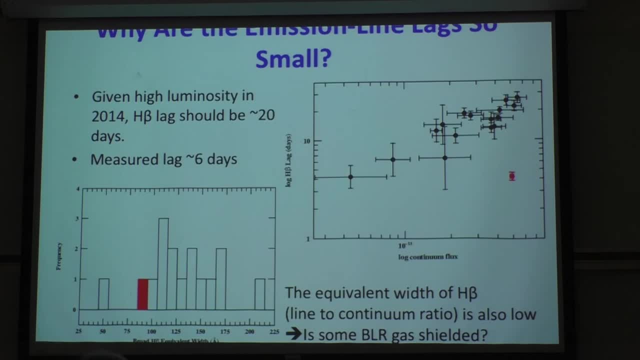 you weren't getting very much line emission. The other thing we found is that the time delay for each beta was much lower, much smaller than one would expect for its continuum state. We would have expected a time delay of about 20 days. 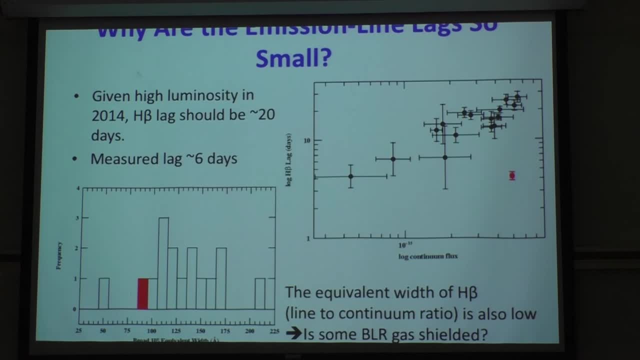 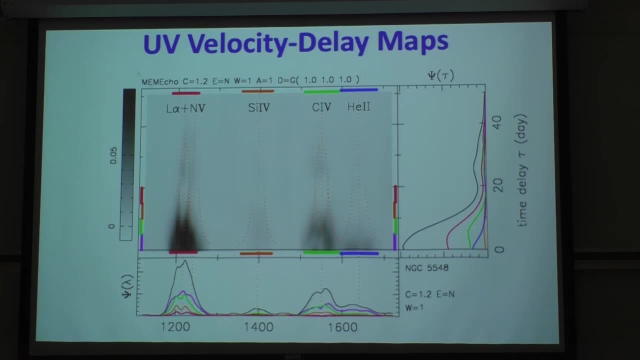 given how bright that it was, and instead we measured one that was closer to five days. So something weird is going on. Okay, let's look at the velocity time delay maps. Okay, these are the things that we set out to recover. 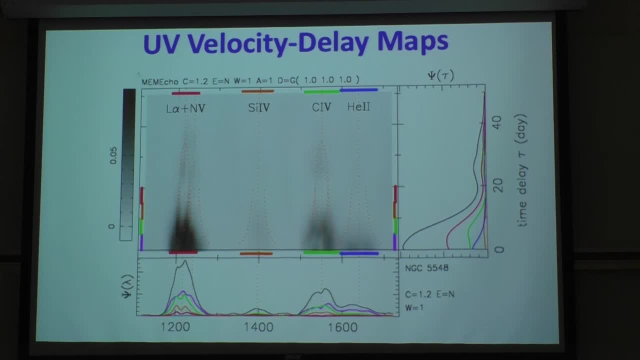 and we do see- which is why I went into this laborious tutorial- about what the disc response would look like. we do see the sign of a disc. we do see a sign of an inclined disc, but it's so faint that we have to actually guide your eye. 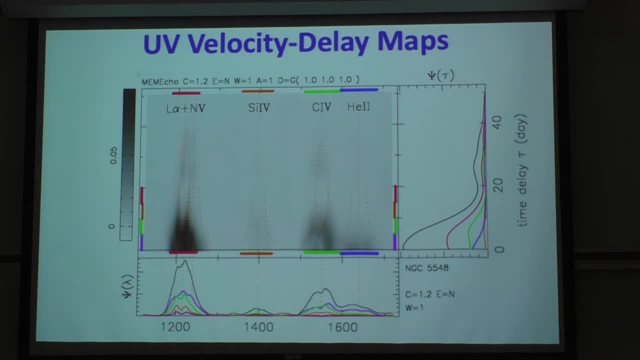 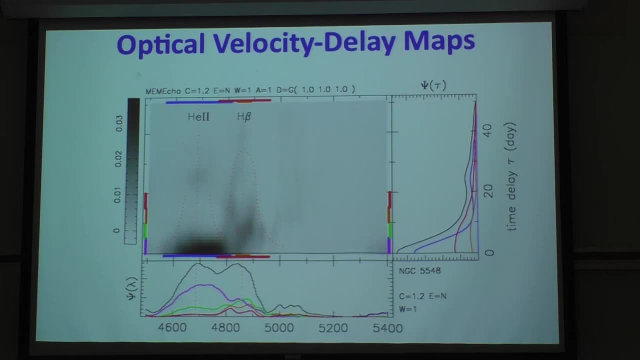 with dashed lines here to show you that there is a disc signature in the ultraviolet lines and also in the H beta, But you'll notice it's very, very weak. The signature of the disc is very weak because most of this actually comes. 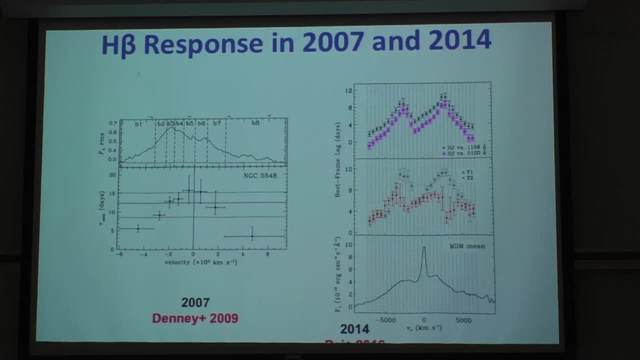 from the far side of the broad line region. So, if we compare this to what we've seen in the past, just in 2007,, for example, this is the H beta response as a function of velocity, and we see as we expect. 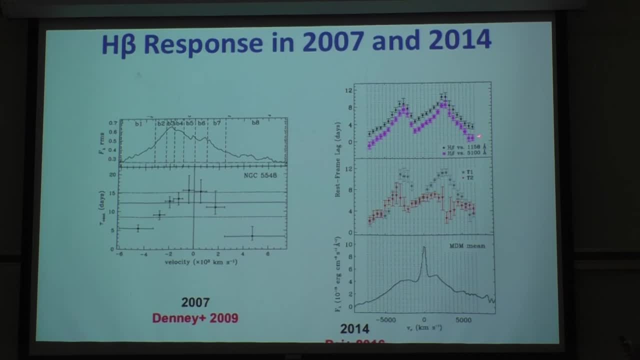 largest time delays occur at the smallest velocities. Here it's very much different. Here we see that there is this hole in the center. We're not seeing the response to the far side, And the hypothesis that we have to explain this is that there is obscuring material on the far side. 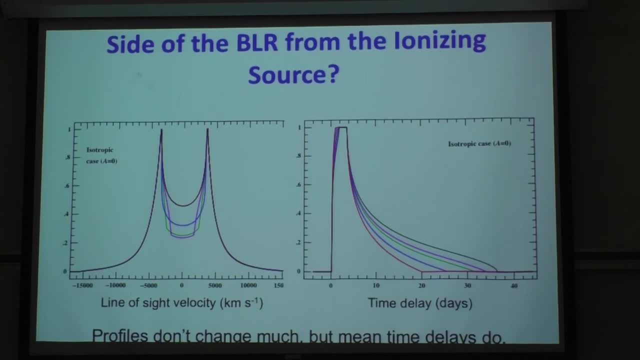 between the continuum source and the line-emitting gas, And you can do this if you. What I've done here is I've just done a series of models where I took a disc that has the characteristics that we have, that we've discerned from the velocity delay map. 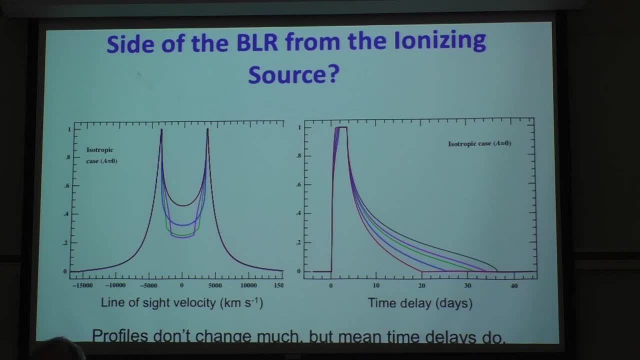 and I preferentially blocked out larger and larger cones on the far side, And if I do this I see that the line profiles don't get too weird. They get a little bit different, But the time delays become markedly slower. The red one is the one where I'm only illuminating. 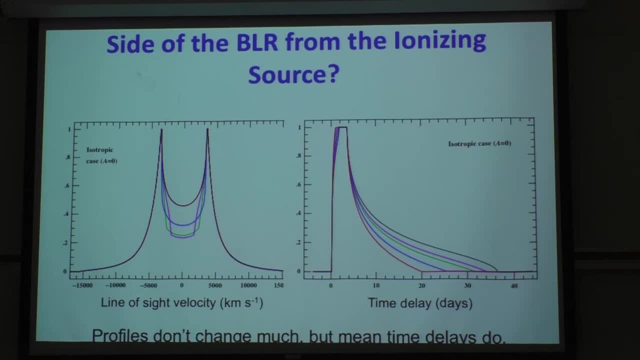 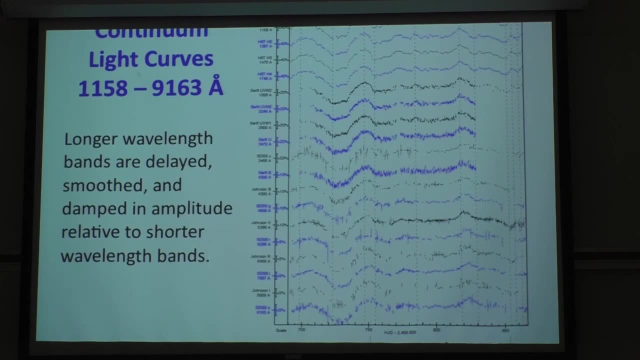 the 2 pi steradians. that faces me rather than the far side, So we can qualitatively explain what's going on here. Another interesting thing that we found out is that if we look at the continuum variations themselves as a function of wavelength, 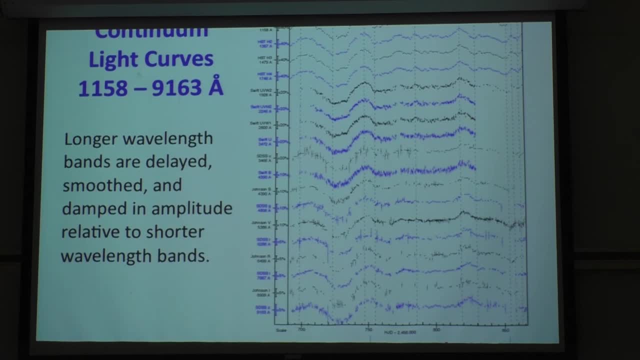 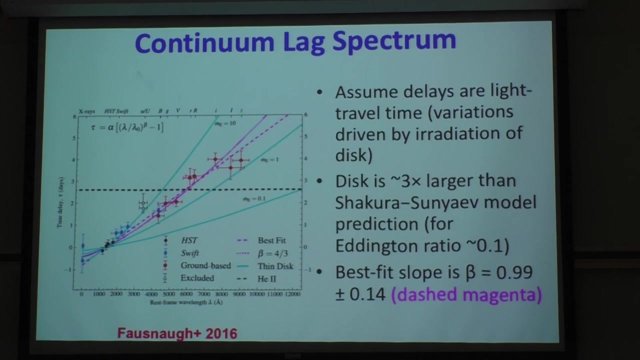 going from the shortest wavelength ultraviolet bands to the longest wavelength, optical at nearly a micron. what we find is that the continuum variations become smoother as you go to longer wavelengths and they are time-delayed relative to the shortest wavelengths. So this is the kind of thing that one might expect. 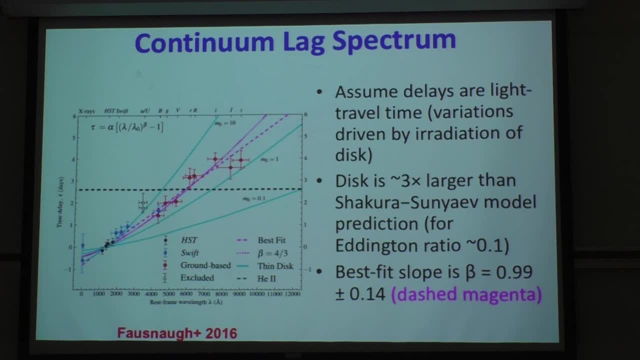 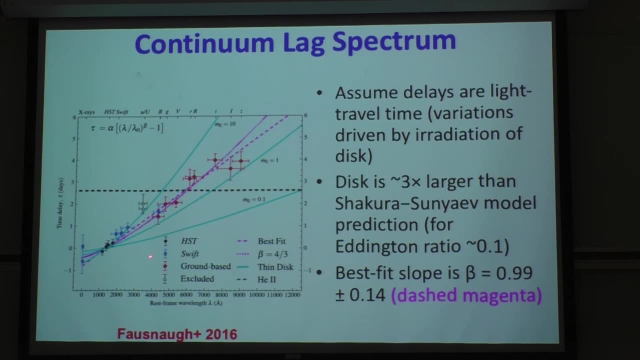 in an accretion disc where you have this temperature gradient And, in fact, the observed points are the ones that you see in red, And the best fit to it is this dashed magenta line, which has a slope of 0.99.. 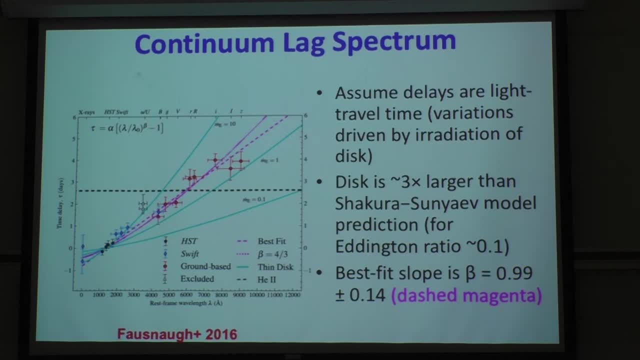 And we would expect a slope of 4 thirds. So it's not terribly off, but it's a little bit flatter than one would expect for a classical thin disc. The other thing is we find that these time delays tell us that the disc is about 3 times larger. 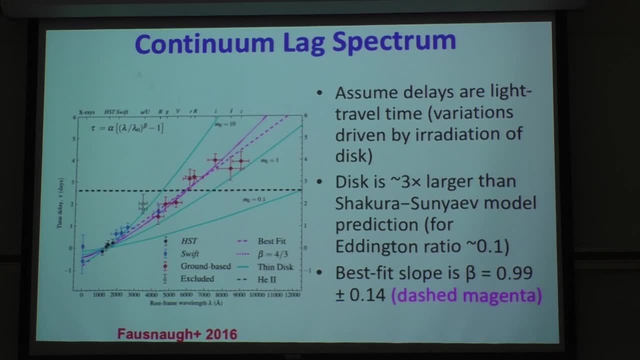 than we would expect for a classical thin disc. We don't know the reason for that. There's a suspicion that we're seeing a strong contribution of the continuum from diffuse emission from the broad-line region That is, recombination radiation that would go from free states. 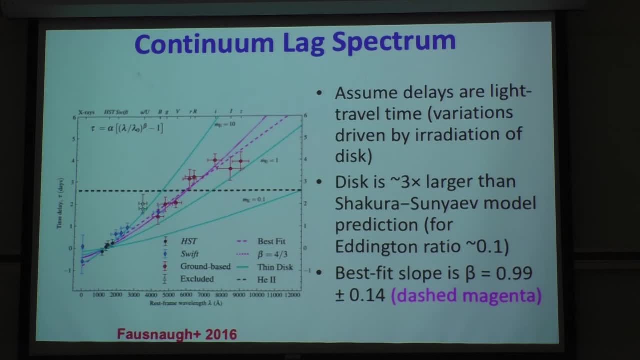 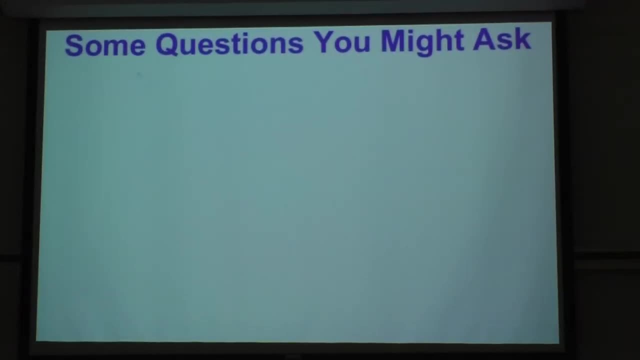 to bound states and emit at wavelengths shorter than 3650.. So that's again something we're in the process of modeling right now. Okay, so some questions that you might ask at this point is: does reverberation mapping really work? 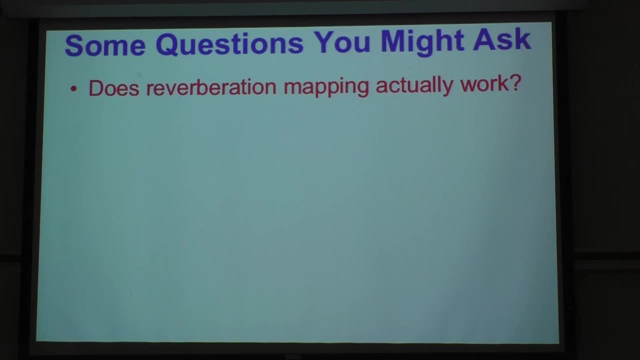 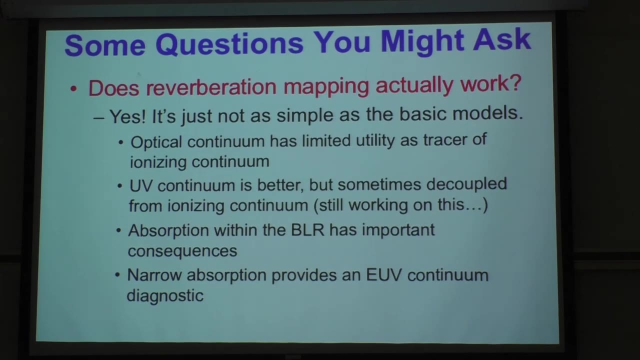 Because we caught this one, AGN, the one that we looked at really closely and really hard And we found that its behavior was odd and we had to invoke some additional properties to try to explain what happened. Well, yes, it still works. 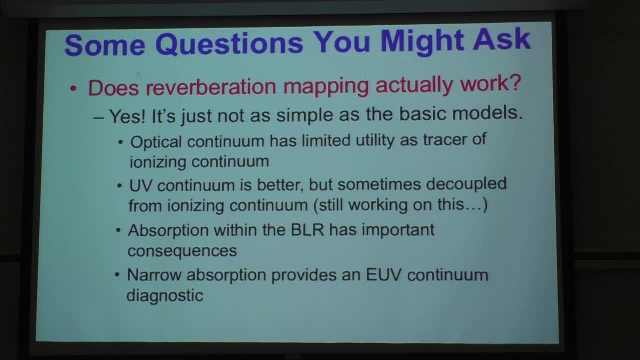 It's just not as simple as the basic models. It's not as simple as I started out explaining to you. We've also seen that the optical continuum has a limited utility as a tracer of the ionizing continuum. The ultraviolet continuum is better. 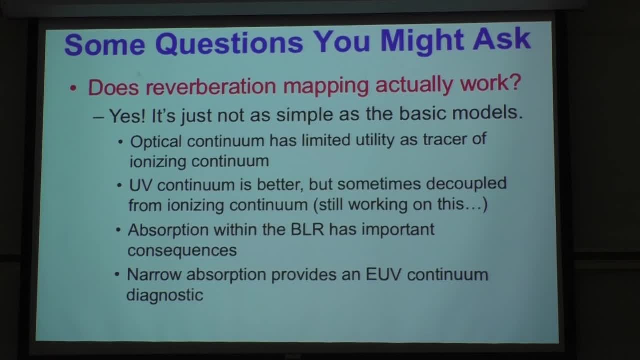 but still sometimes decoupled from the ionizing continuum, And this is a complication that I did not bring up because I'm running out of time. Absorption within the broad line region has important consequences, And something I didn't get a chance to talk about. 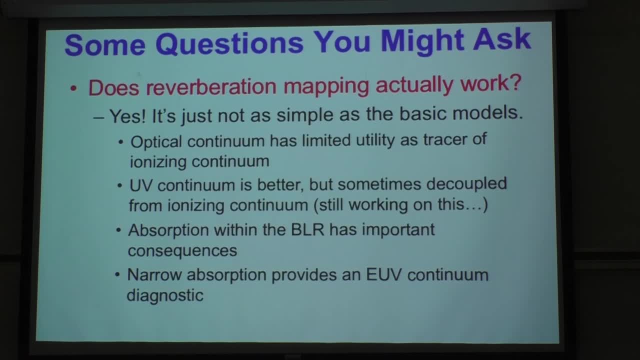 because, again, for lack of time, the narrow absorption lines actually provide us with an important continuum diagnostic, because they are observing the same continuum that we are. This absorption occurs along the line of sight to the AGN. Okay, so you might say: 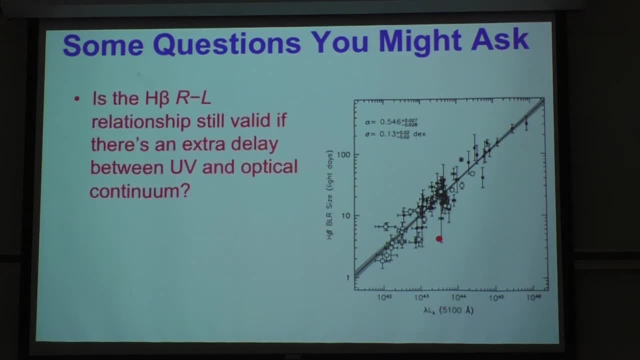 is this H-beta radius luminosity relationship? is this still valid? Because we found this one point that was way lower than it should have been, and this is where it would project on the diagram that I showed earlier. So what we're seeing? 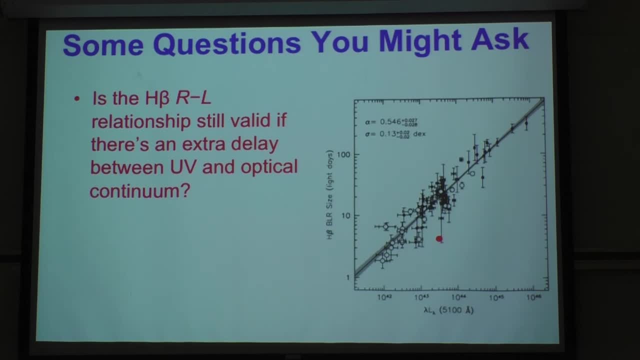 sometimes you catch objects in transition And that's what we think we're seeing here. We're catching an object that has been transitioning from a state where it was almost off and we think what happens is basically the broad line region collapses When it turns back on. 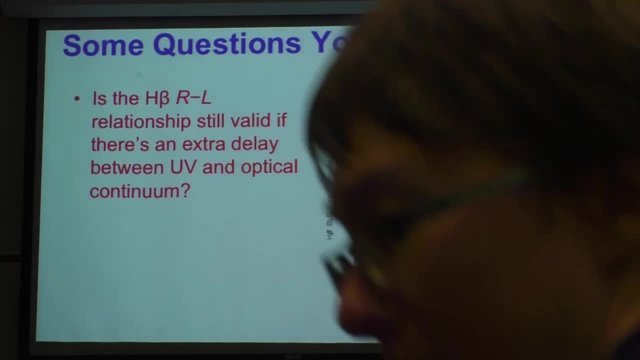 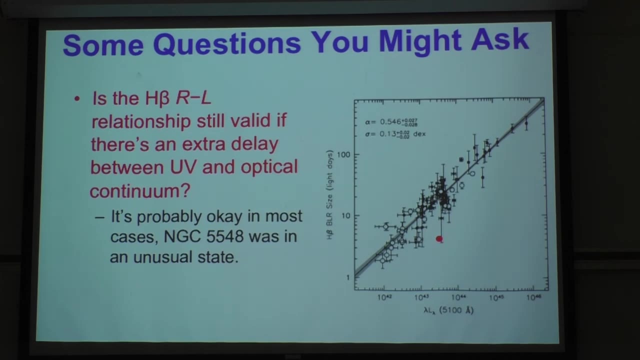 it takes a while for things to stabilize. That's fundamentally what we think was occurring, But we would have probably noticed that this is an outlier and that we caught NGC 5548 in an unusual state, While it was in an exceptionally luminous state. 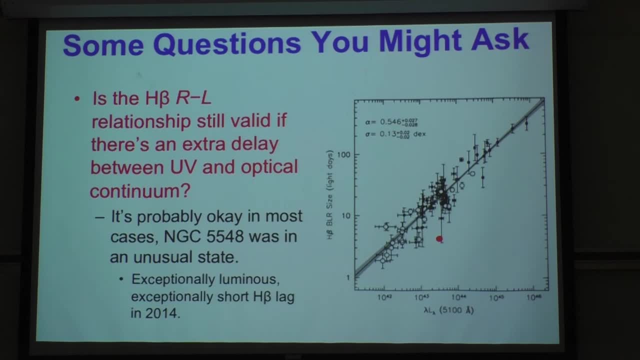 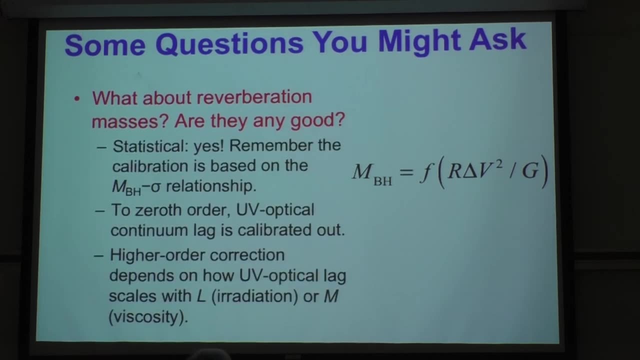 we found that the H-beta lag was also exceptionally short. So what about the masses? Are they any good? And statistically, yes they are, Because, remember, the calibration is based on the M-sigma relationship and that takes out any bias here that we might have. 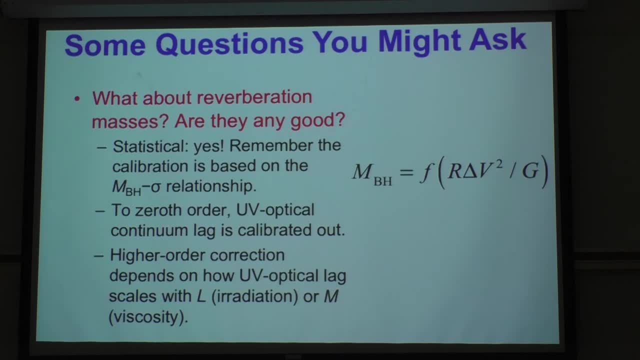 because we're looking at the optical continuum lag and we know that that lag is behind the ultraviolet. So there's a correction factor that needs to be put in there. but to first order, this correction, factor F takes care of that And let's see. 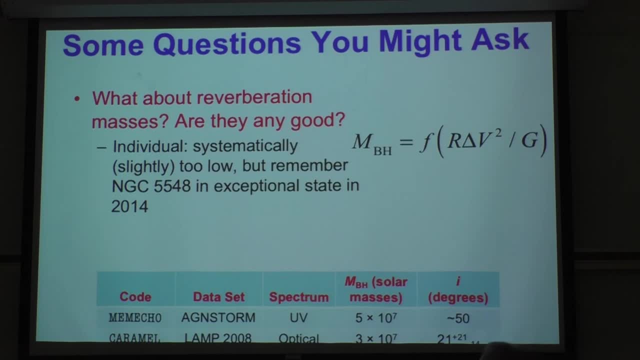 Yeah, the individual masses, however, are systematically slightly too low, but remember that we're looking at NGC 5548 in an exceptional state. If we look at two previous measurements of the black hole mass and compare it to the one that we got, 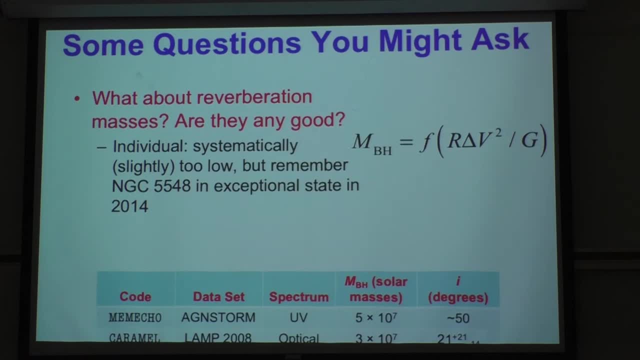 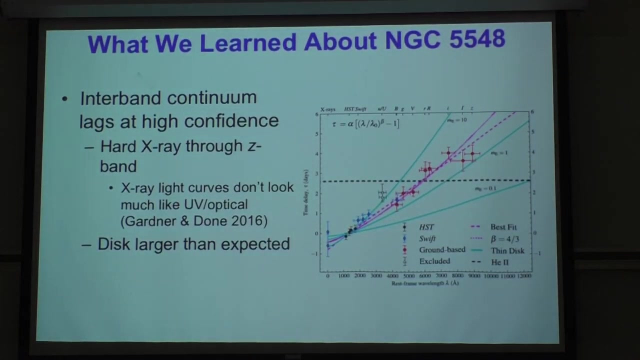 from our AGN storm campaign. they're close enough Because, remember, any individual measurement is only good to a factor of three or four. So nevertheless we see reasonable consistency there. So things we learned about NGC 5548 in particular. 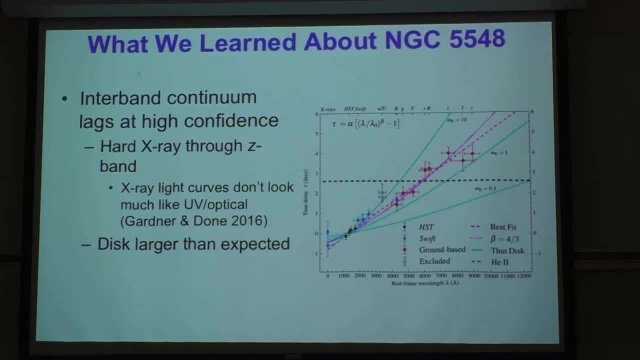 we learned about these interband continuum lags and they were detected at a high level of significance really for the first time. We also see that the hard X-rays don't look very much like the UV optical, So we've got some explaining to do. 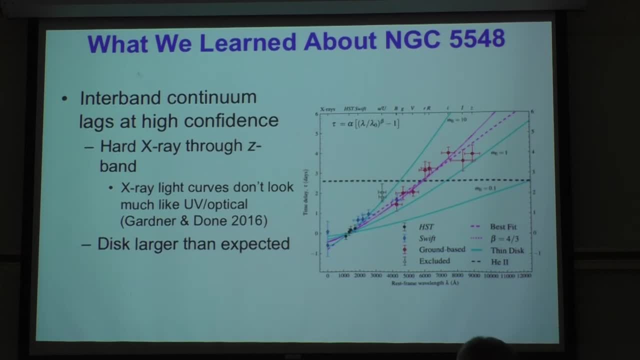 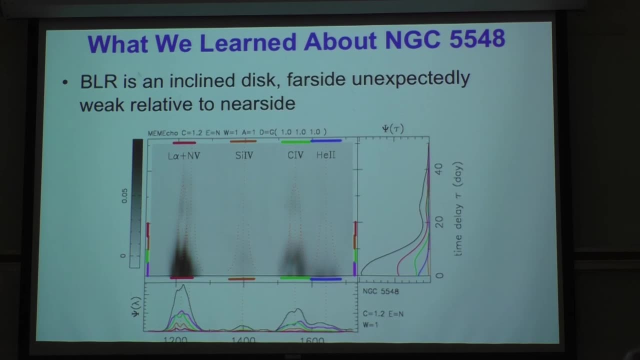 about where the X-rays are generated and how. We found that the accretion disk is larger than expected. We also found that the broad line region is an inclined disk and the far side is unexpectedly weak relative to the near side, possibly due to some obscuration. 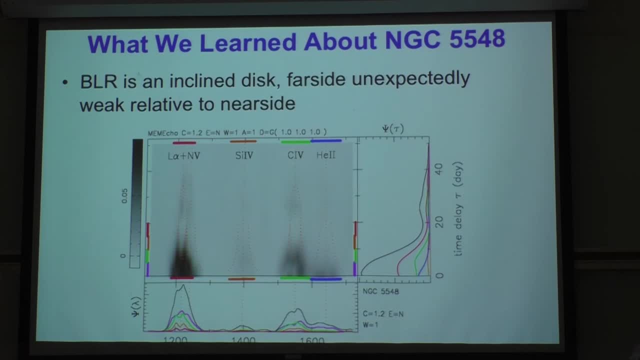 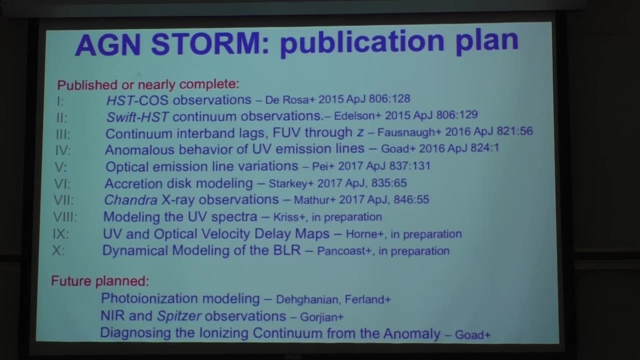 that occurs between the continuum source and the line emitting gas on the far side of the region. So this is kind of a progress report. We're still trying to figure this out. We have currently published seven papers on this. We have three more that are in preparation. 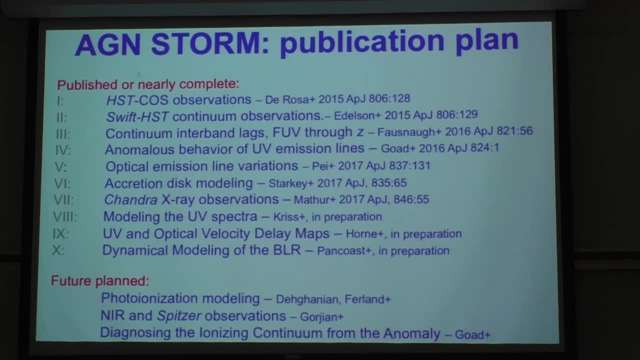 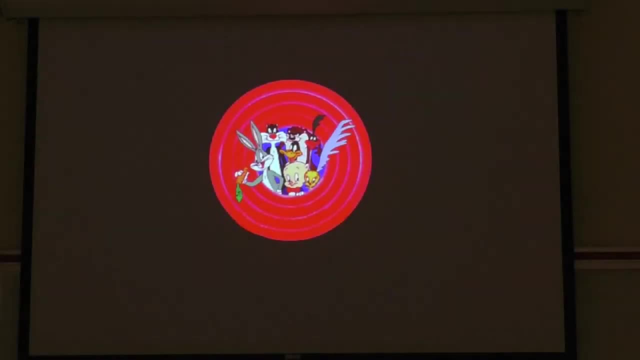 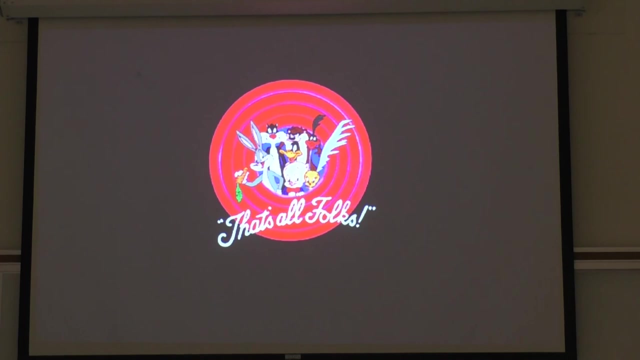 and at least another three that people are working on right now and expect to have additional results within the next year or so. So at this point I will stop and be happy to take any questions that you have. I know we kind of drank through a fire hose there. 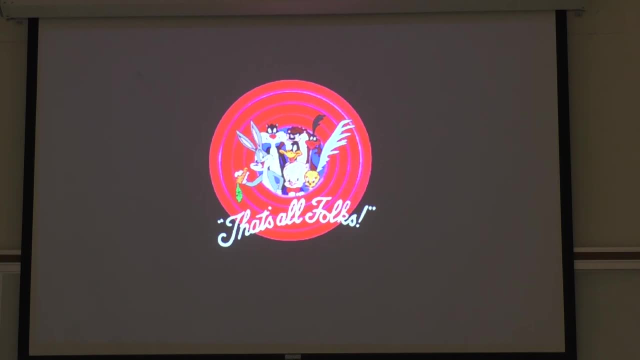 so I need to go fast: The creation of the broad line path and thinking of how they're created, how long they're created, how long they are able to survive and what happens, say, when the NGN, the continuum source, does turn off. 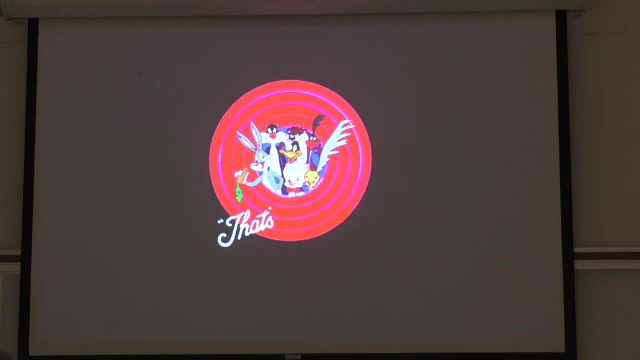 Are they blown away? Do they evaporate, You know? do they just sit there because they're unable to do anything? Well, I kind of think of them rather. you know, we use clouds as kind of a device, but I tend to think of them as streams. 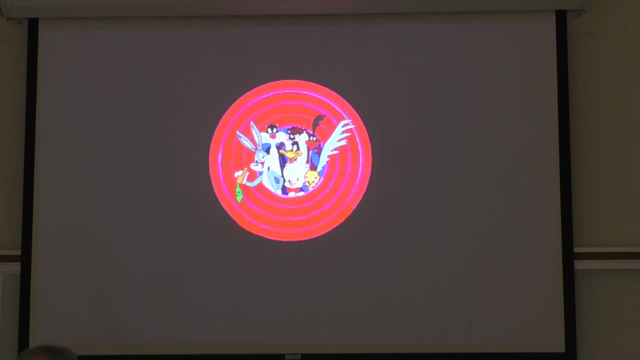 because they're dynamically unstable. But I think that what we're seeing is inflowing gas from the molecular torus and this is what piles up and essentially, the broad line region is an outer extension of the accretion disk. It's the dynamical models that people are doing. 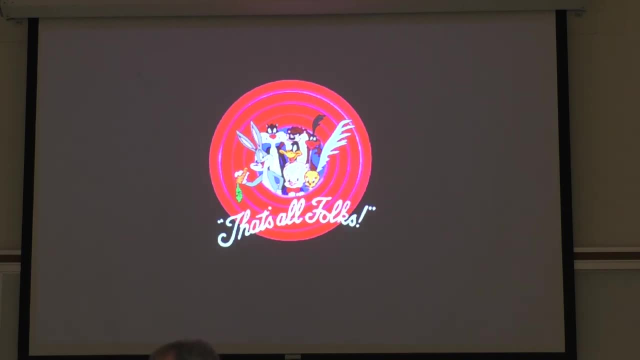 and the thinking of these regions show that they are not thin disks, that they're rather fat disks, and you actually need that to intercept enough of the continuum radiation to get the amount of line radiation that you see. So I think that the situation is very dynamic. On the half dozen or so, I think it's maybe up to ten now- AGNs, which have gone one stage further than this and done dynamical models. you always seem to find evidence for a fat disk and sometimes you find evidence for outflows. 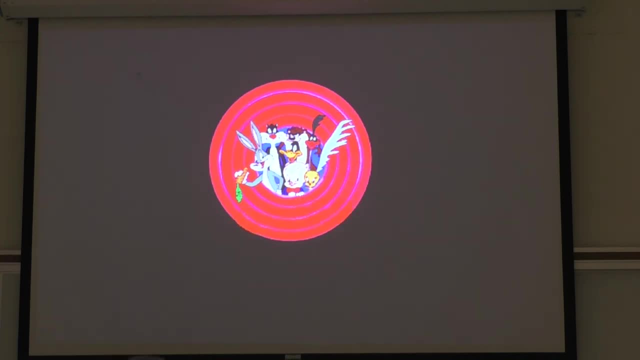 and sometimes for infall. So there's a lot of stuff going on. Basically everything that can go on happens Just for this audience. what's the angle of this When you say fat, When I say It's almost torus-like itself? 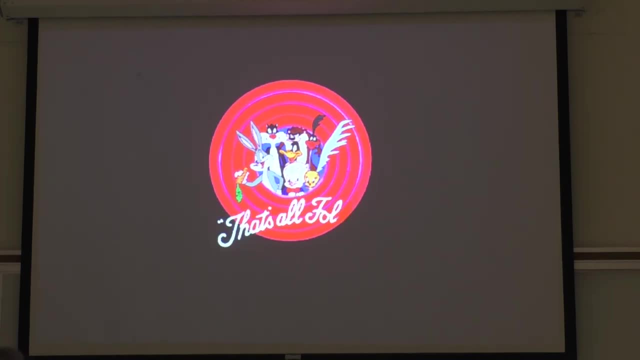 I mean, it's not like it gets larger with increasing radii, So like 45 degrees from the center, Yeah. 30 to 45 degrees, Yeah, Okay. So this broad line region is less than a parsec from the center of the particle. 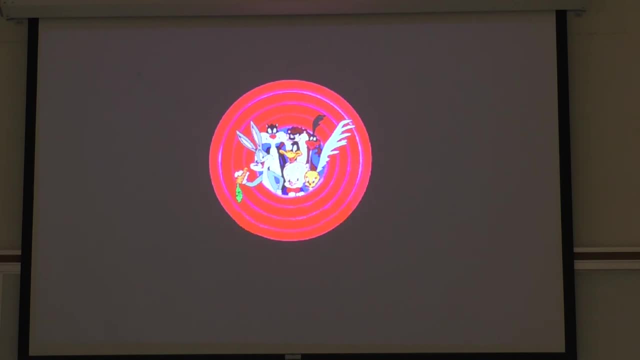 Yeah, Yeah, That's a few light days, So a hundred days. and where does it start? So it's inside the bulge, like way inside the bulge of this galaxy. Are there any effects, like absorption effects and all this? 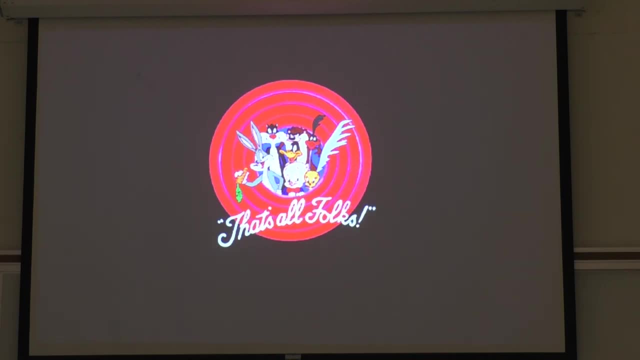 They're attributed all to this model. but this model is inside the bulge of the galaxy. So you're looking through. All your observations are looking through the bulge, maybe part of the disk. Are there any effects that you attribute to? 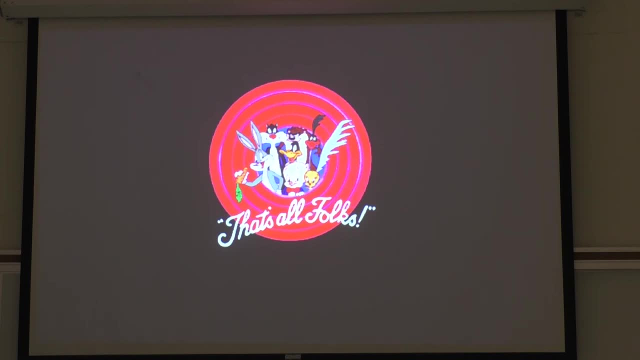 You have to correct for the host galaxy. Well, yeah, I mean you can see the contribution of the host galaxy starlight in the spectrum And the way we estimate that is, we get high resolution pictures with Hubble Space Telescope model out the central point source. 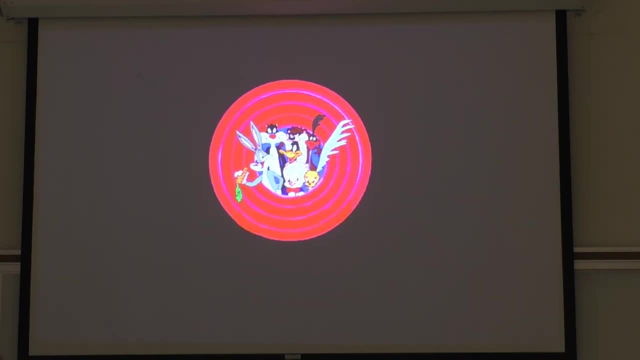 and then that gives us the starlight distribution, And we then perform what we call simulated aperture photometry. We put essentially our spectrograph entrance aperture on top of that and see how much starlight there is, And we subtract that off our continuum measurements. 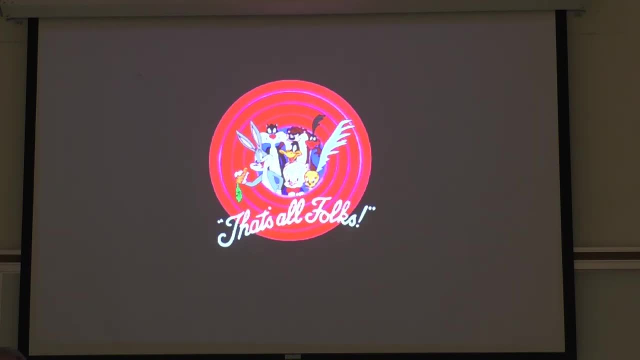 So now, in terms of physical effects, this is one of the hot topics in quasars right now. There are, There are in large galaxies. Large galaxies stop star formation before they should. There should be more massive stars than there are, And the question is: why does this happen? What stops star formation in galaxies- And one candidate is quasar activity- that it basically heats up the interstellar medium to the point that it either blows it out or it just makes it so hot that stars can't form. So that's an area of active research right now. 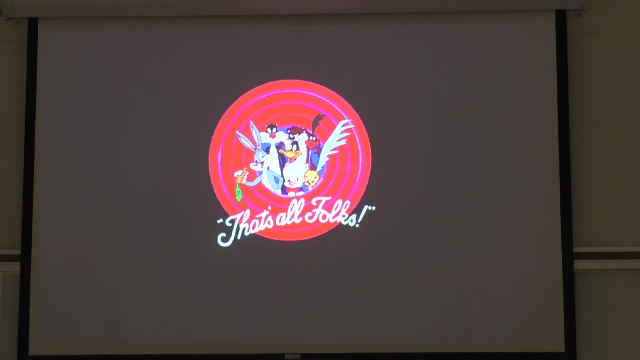 that's been active for 10 or 15 years and without suitable resolution. Things take a long time in astronomy. You can say something about the origin of the clouds by the metals that you're seeing. right, You're seeing It looks like interstellar medium. 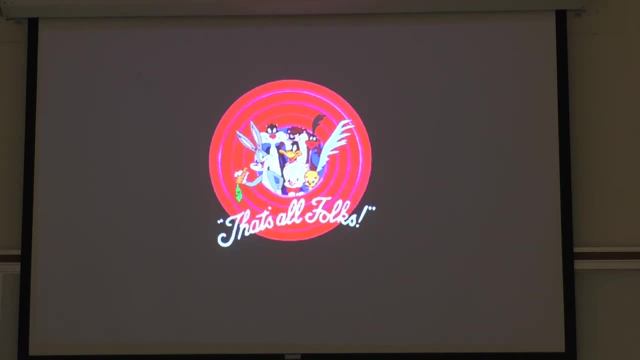 almost exactly like there are clouds in a population more than 400 million stars. Well, yeah, the. The problem with quasars in some sense is that. Well, first of all, it's hard to measure abundances from an emission line. Much easier with absorption lines. But it looks like even in the most distant quasars the metallicities are approximately solar, So at least in the inner parts of the galaxies you're seeing formation of metals very, very early in the history of the universe. 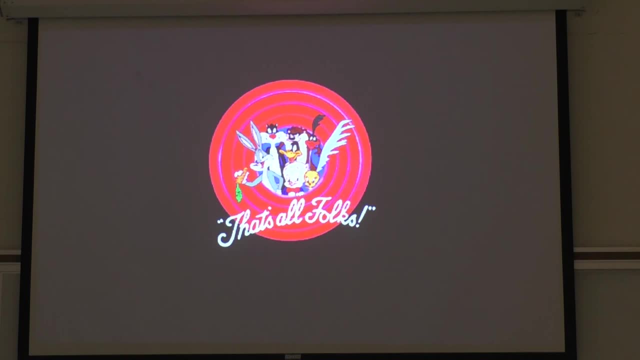 So, again, that's something else that we don't understand. yet I didn't mean to imply that, Yeah, the ultraviolet, Yeah, the ultraviolet that we see is arising from the accretion disk, And it's. It varies in the same fashion as the optical continuum. 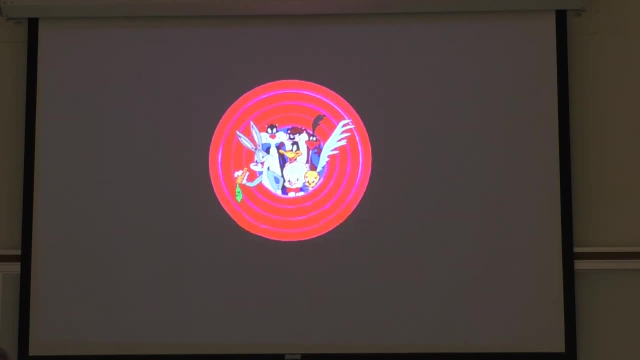 though the optical continuum is a smoothed and shifted version of that ultraviolet continuum. So something is: Whatever is driving ultraviolet variations is also driving the optical variations. Uh, if you can convince the HT tag to give me another 176 orbits to observe the same source or a different one. 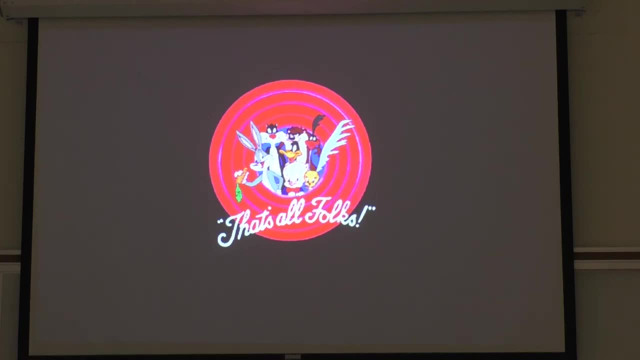 Boy that's. I lose a lot of sleep at night wondering about that. Um, Uh, I think. I think you know the only way I could get away with doing this one again is if they gave me enough time to do five or six. 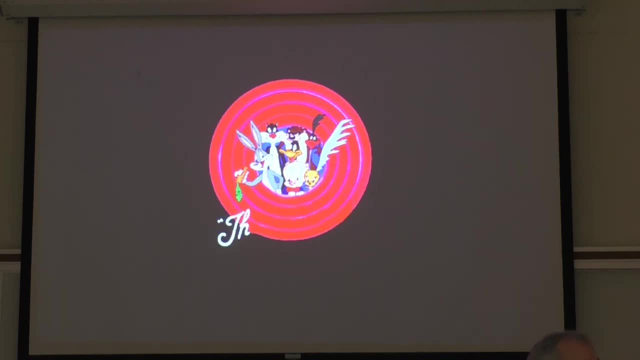 Then I would do this one again. But you know, I think if I asked to do this one again, they'd say: you're kicking a dead horse. You know we're not going there again, But you know we will try with other sources. 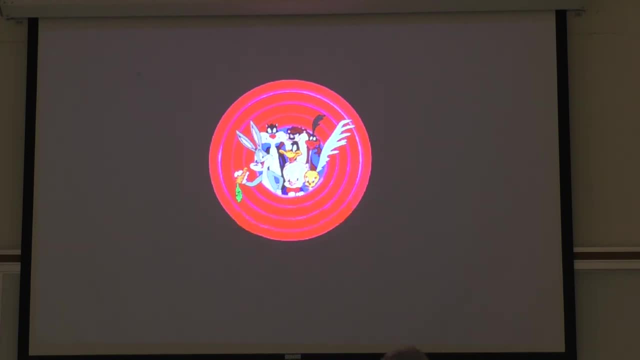 We're, uh Um, Not too long from now, say around 2024,, we're not going to have ultraviolet spectroscopic capability in space anymore. So if this really works for you know, discerning how the gas is moving, 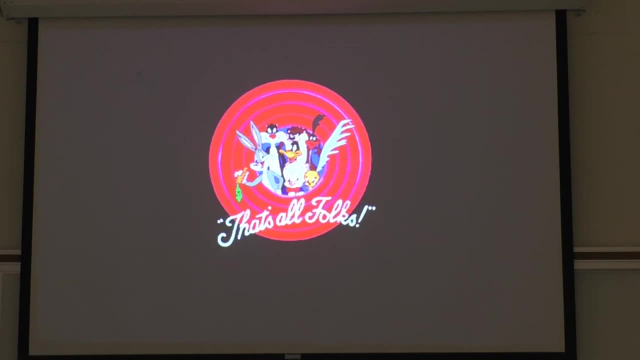 we need the ultraviolet, and we either need to do this before Hubble dies or we need to invest $200 billion in a single-purpose, small ultraviolet telescope that can do that, And they can do this all the time. Neither of those seems particularly likely. 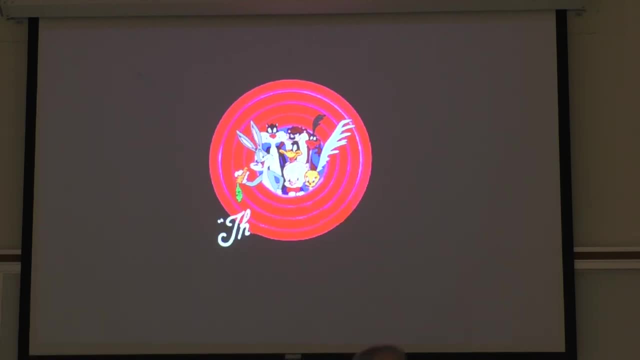 So we will continue to knock on the door at Hubble with, um, You know, with sources that we consider will remove some of the ambiguities that we have remaining from this program. Oh, yes, and we continue to do that. So, uh, 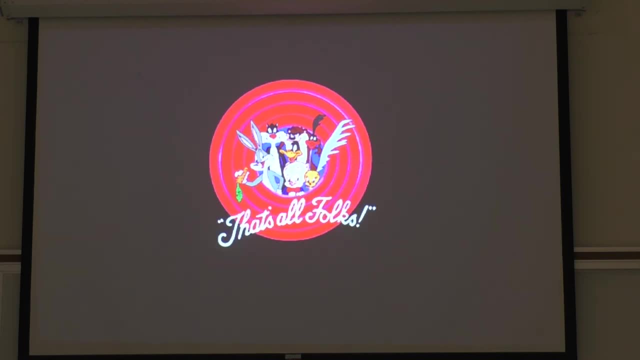 If you want to know what the high ionization lines are doing, you do, yeah, And the other thing we have to try to understand better is the delay between the ultraviolet variations and the optical variations, And are they correlated? Is that delay correlated with luminosity?